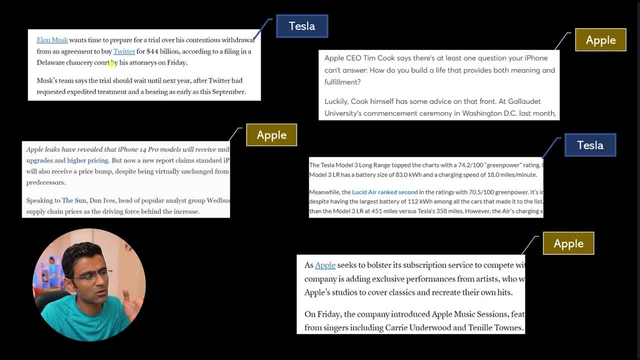 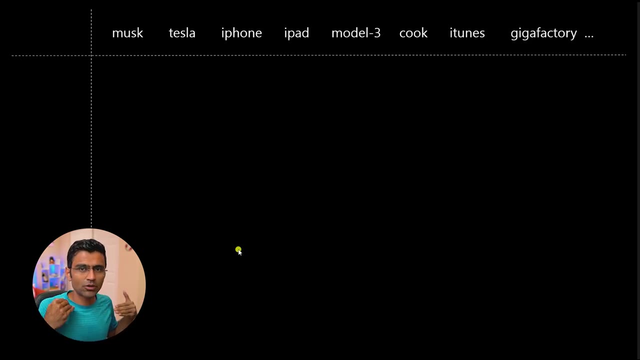 know that this is about Tesla, And when you encounter terms like Apple, Tim Cook, iPhone, iPad, you know it is about Apple company. So one way you can auto extract the company name is by building a vocabulary. So the vocabulary may look something like this And then for each of these articles you can have a word count. For example, I have some random 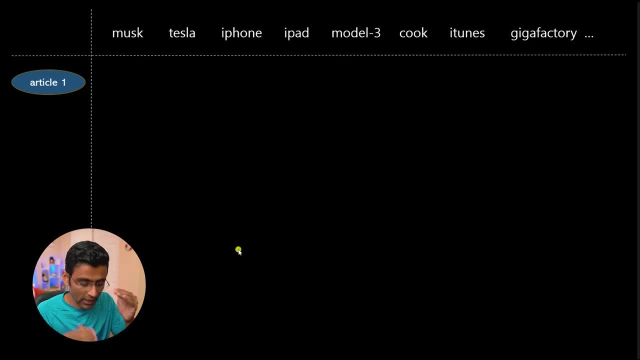 article I can put. I can go through the articles- Okay, I can, and then I can do a word count. So the word Tesla appeared 14 times in that article, Model 3 appeared nine times. The remaining words were zero and Gigafactory appeared two times. This way you can just get a simple word count. This is no rocket science. You're just counting the words. You know this word appeared how many times in the article And at. 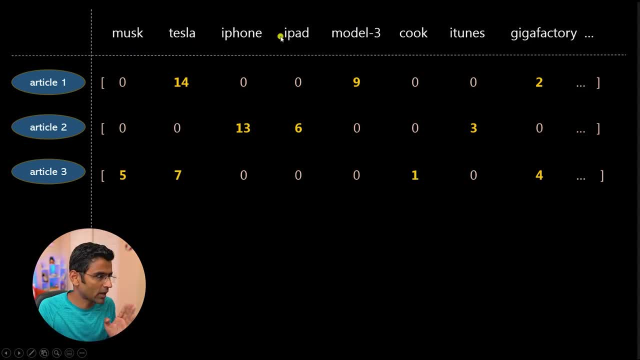 the top, you have written the entire vocabulary, and by vocabulary i mean, let's say you have 100 articles. out of those 100 articles, you will take unique words and you would probably apply some stemming lemmatization and you will create that vocabulary. it could be, let's say, 10 000 words. okay, 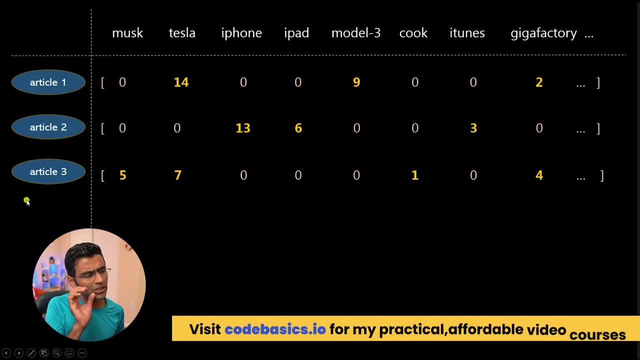 and if i give you these vectors, right, these numbers, sequence of numbers, are nothing but vectors. if i give you these vectors, just by looking at this vector you will be able to tell me that this article is for tesla, correct, because see the word tesla, model 3 gigafactory, came. 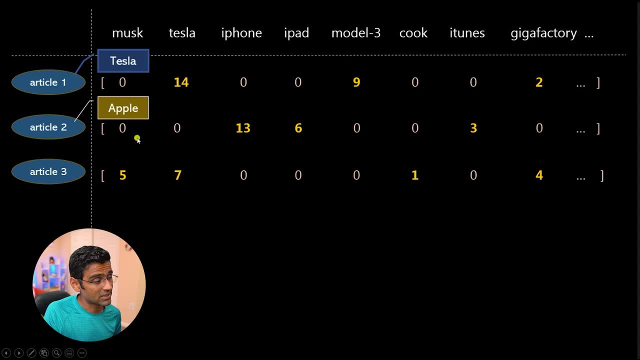 multiple times. and the other article is for apple, because iphone, ipad, itunes, this kind of terms were present. the third one is for tesla. again, musk, tesla were present. there was a cook tim cox reference in the tesla article as well. it's possible, right, because the news articles are talking about competition and such 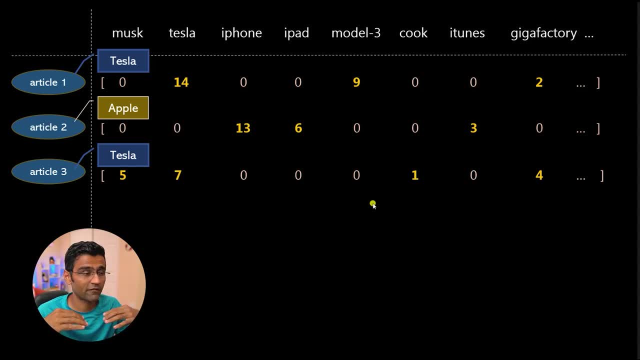 so it's possible that you will see some references of terms which are not related to tesla, but it could be related to some economic conditions, competition and so on, and that's fine. but overall, by getting a frequency of the words, you will be able to tell what company is this and this is bag. 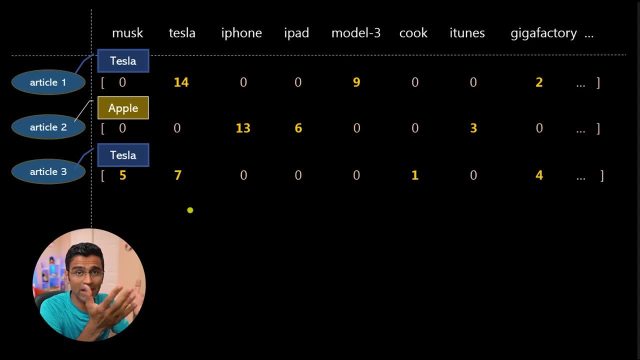 of words, basically for bag of words. this is a bag of words- numeric representation. all you do it is you have a vocabulary, you get the word count for each of the words which are present in the document and you create a vector and that vector is also called count vectorizer. you know when we'll use. 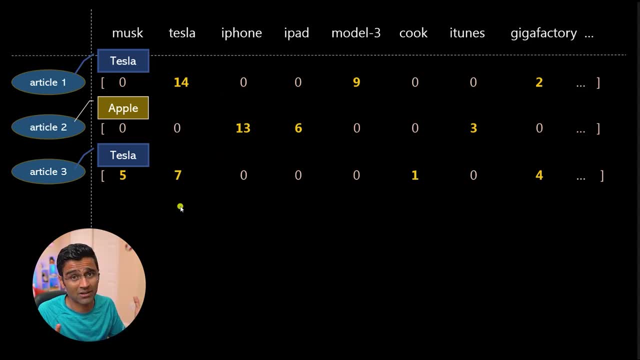 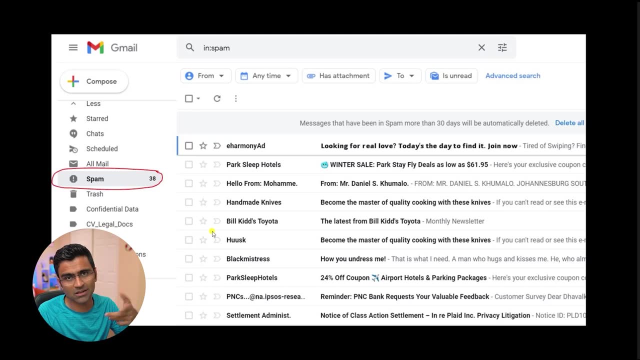 a skill on. we'll come across this class called count vectorizer. now we are doing, going to do some, and in that we'll be tackling a classical spam problem. right, this is. this is an image of mark, the real gmail screenshot that i have, and gmail is very good in terms of detecting spam. 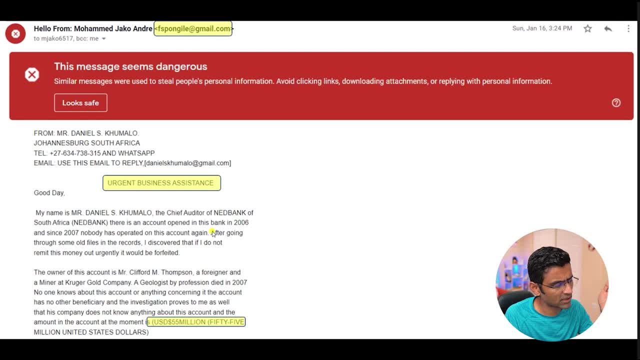 um, i have, i got this email and in the email, just by looking at the term, such as you know, i have 55 million dollars in my bank, for example, origin business assistance. so just by looking at these way, uh, these terms, you can tell that this is a spam. 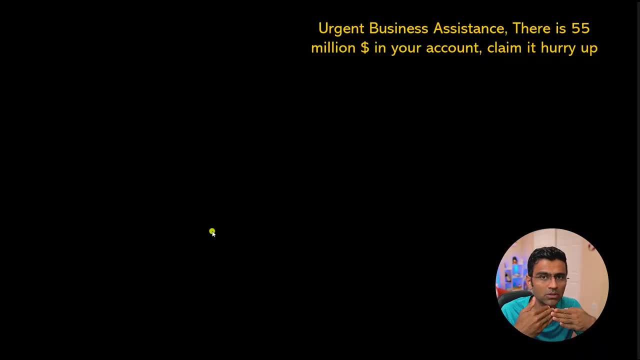 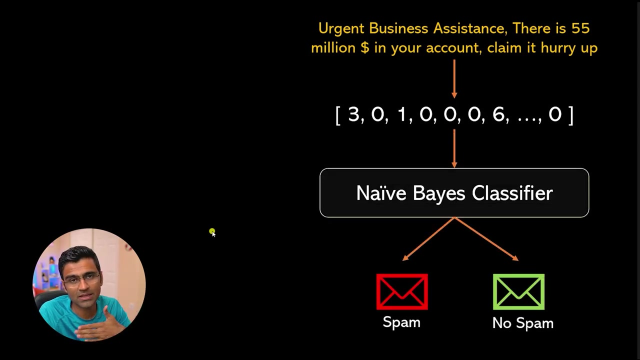 so the model that we are going to build in today's tutorial. we will take an email body, we'll convert that into numbers using bag of words model and then we'll apply naive Bayes classifier, which is one of the classifiers in a skill on. there are many classifiers: naive Bayes, random forest. this is entry. 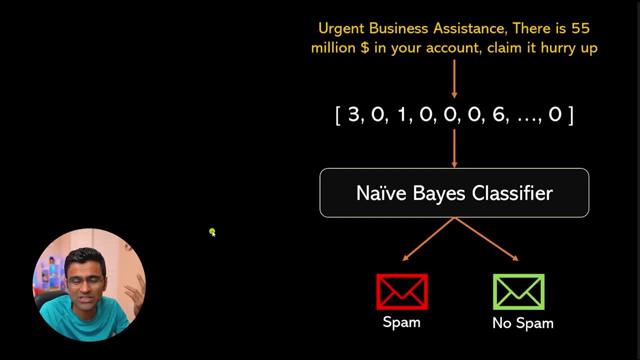 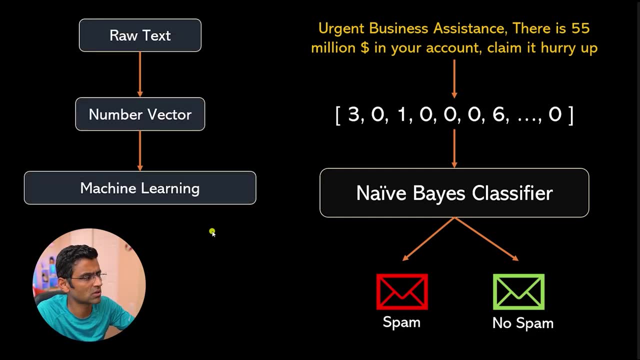 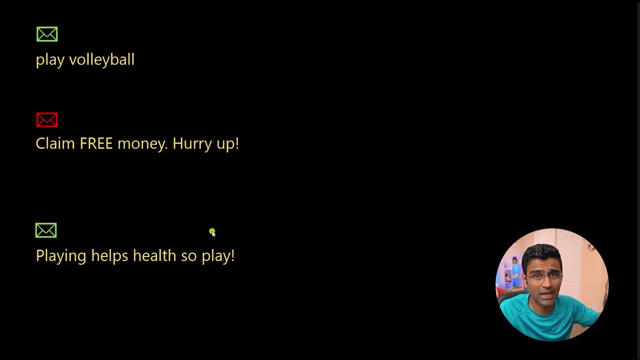 and so on. we will be using maybes- you can you try other ones as well- and measure of performance. so the abstract approach we are taking here is: we have our text, you're converting it to a number vector and we are doing machine learning on top of that. so I'm going to go over this approach when we have all 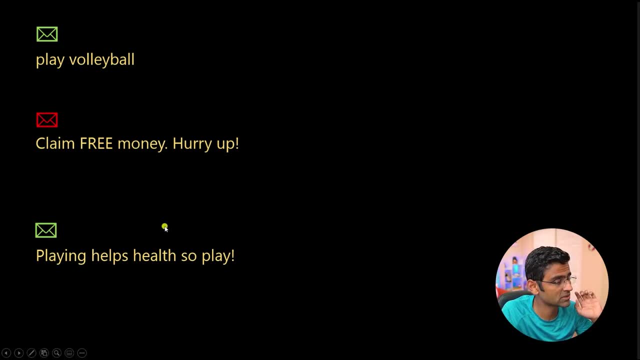 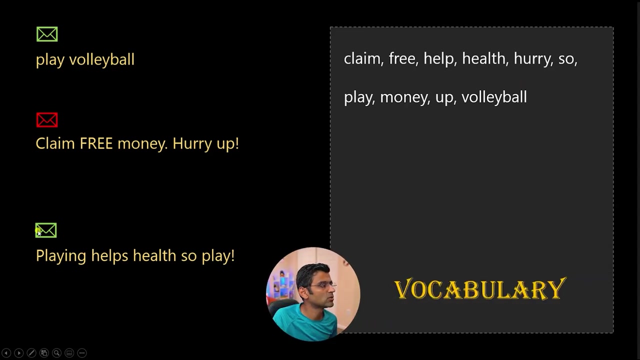 these emails. you know the middle one is a spam email. the other ones are not spam email. we will be building a vocabulary. first vocabulary is a unique count of words in all your emails and that vocabulary looks like this: see, this covers all the words that you came. 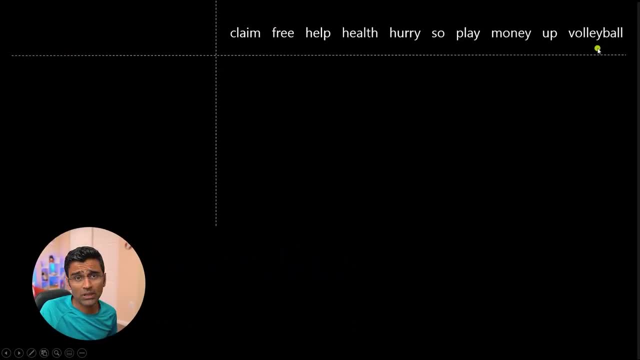 across in these three emails and then we will build a bag of word or count vectorizer where we take an email: okay, this is one email and we put a count. so play came one time, volleyball came one time. I played volleyball for two hours this morning, by the way, and here for example, playing and play, so playing if 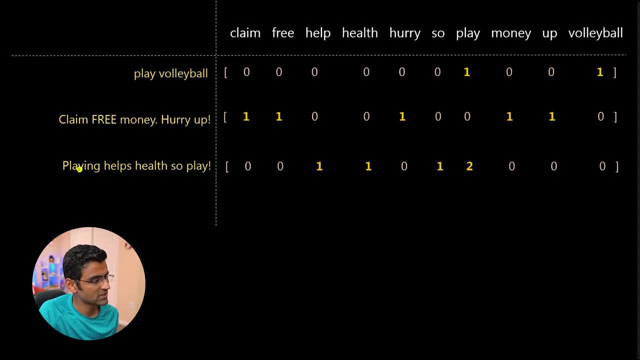 you do stemming, playing will be reduced to play. so you can say: play came twice right here and here. so therefore in the play I have two times, so cam one time and the remaining word cam zero time. so this is the bag of words presentation model for this particular text. 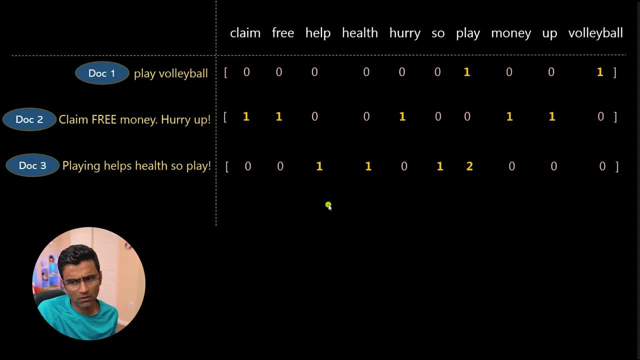 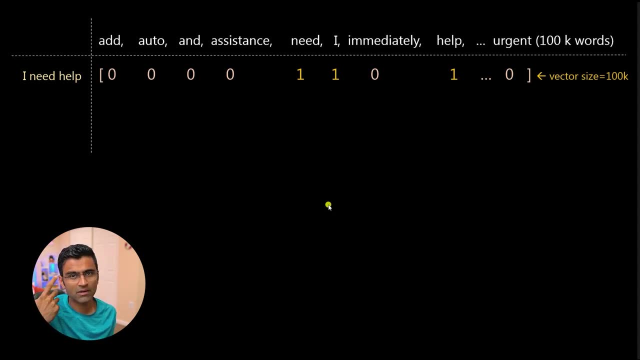 all right now there are certain limitations of bag of word model that I want to discuss quickly, and you already noticed that your vocabulary could be long. plus I have a hundred thousand words. you know I have those many emails. then each vector for each email would be of size hundred K. this is still better. 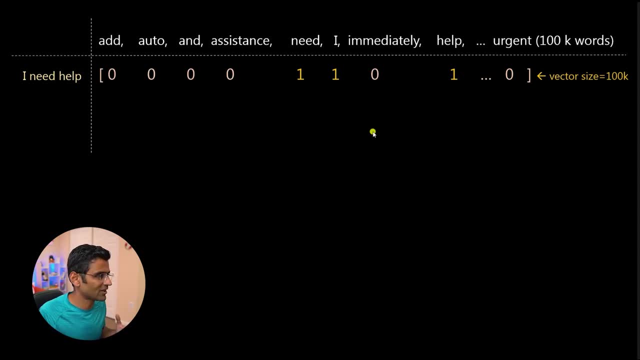 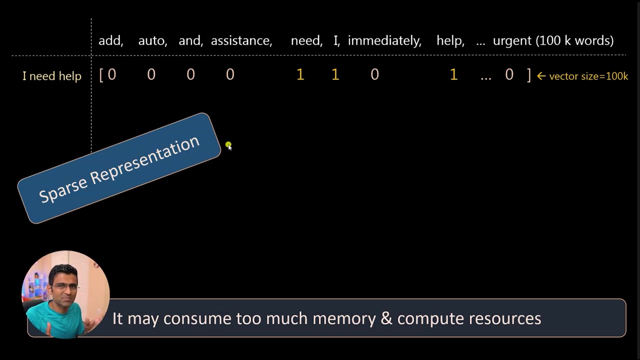 than one hot encoding, because in one hot encoding one word itself will be hundred K. here the entire email would be hundred K. okay, so it is, the size is less than one hot encoding, but still it is. it is a sparse presentation, basically. sparse presentation is basically: you have a big 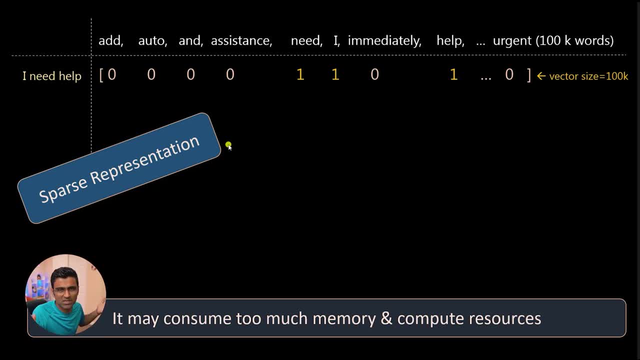 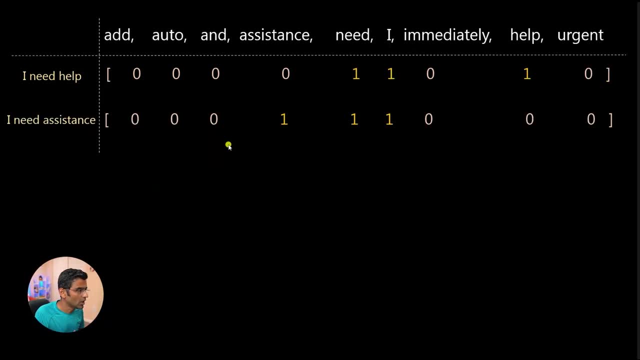 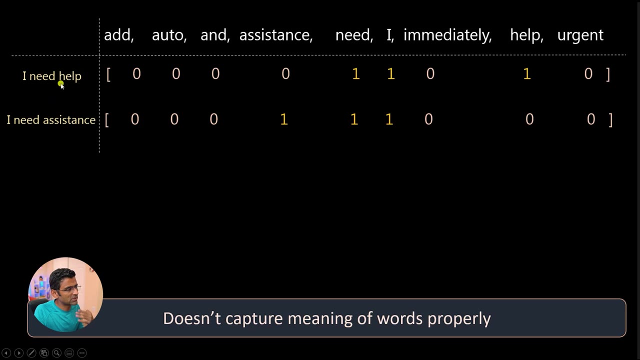 vector where most of the values are zero. that's called sparse presentation, and this consumes a lot of memory in computer sources. so that's, this is number one. the other one is it doesn't capture the meaning of your sentence accurately. you can have two emails. I need help. I need assistance. 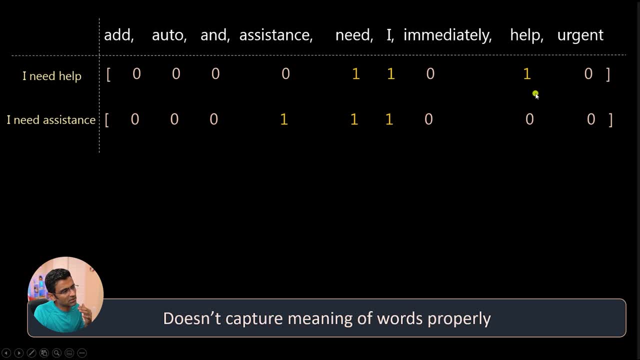 help and assistance are kind of same, so that I expect that the numeric representation of both of these emails is similar. but no, here we are just having one word as unique word and we're just doing a count. you know word count. therefore, the numeric representation of both of these emails is different, see: 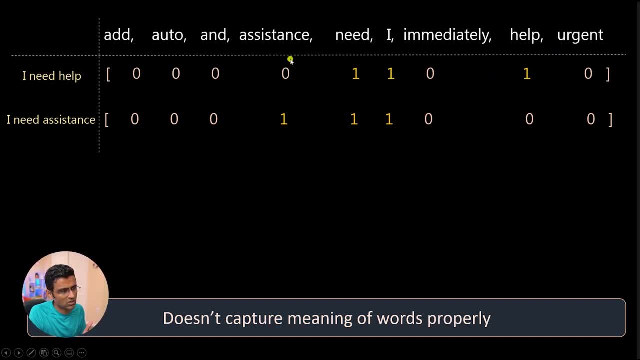 here we have one one, one here. here you have zero and one here, so they're different. so it doesn't capture the meaning of words properly, but that's okay. in today's coding you'll see, we'll be able to get pretty good accuracy with the bag-of-word model and, without further ado, let's start writing the. 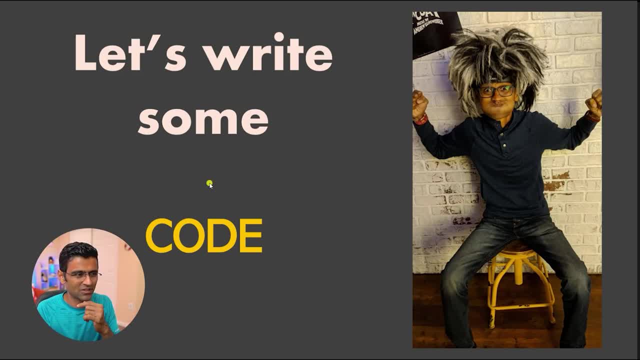 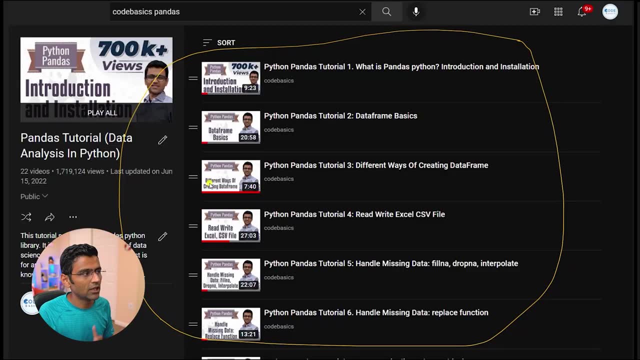 code- and, by the way, this is me in the picture here. so we're going to write the code. and before we write the code, there are some prerequisites which I have mentioned before as well: that you need to know Python first of all. you need to know the pandas if you go to youtube codebook. 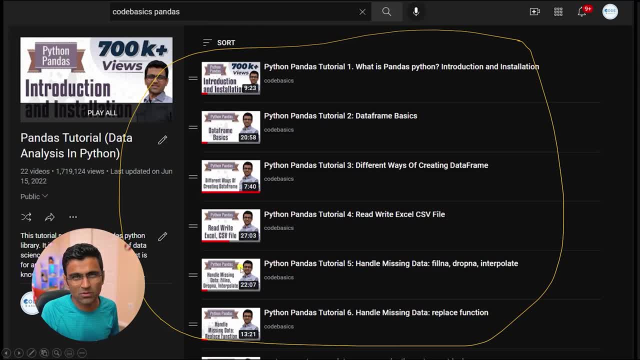 you need to know the pandas. if you go to youtube codebook, you need to know the pandas. if you go to youtube codebook- basics, pandas- I have tutorials you follow first. seven or eight tutorials in pandas is good enough. and I have machine learning tutorial playlist again here. 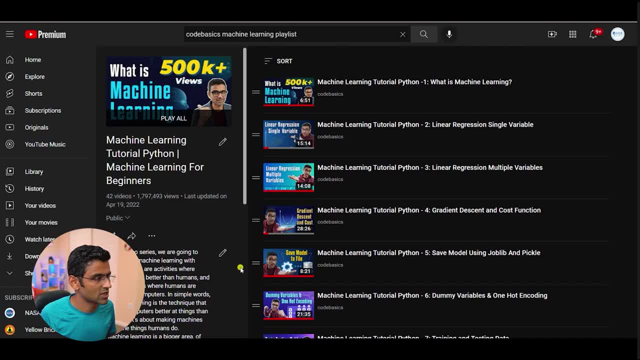 you can follow maybe first 14 or 15 videos and you will have some good understanding of how to use scikit-learn, train, test plate, things like that, and we are going to use all of those concepts in the coding part today. so we are going to do some coding and in the end we'll have an exercise for you as. 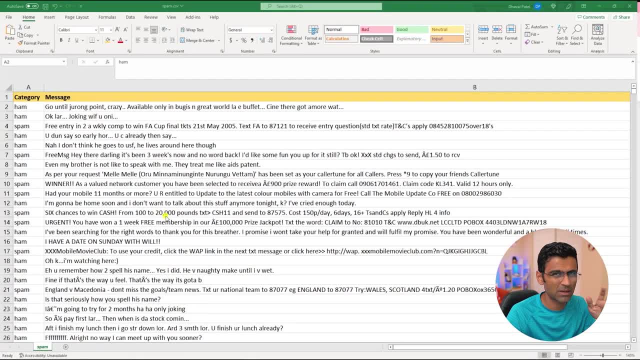 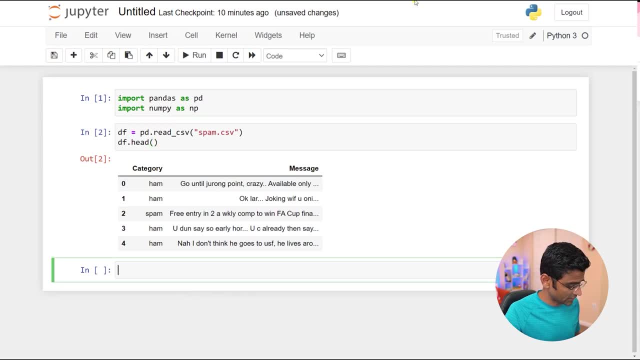 well, I have this data set of spam and non spam email. more than 5,000 email which I have are loaded in my pandas data frame and the first thing I will do is I just try to figure out how many spam and non spam emails are there and in pandas data frame on a series. 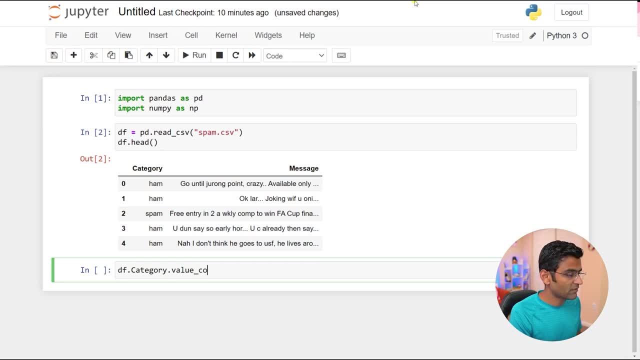 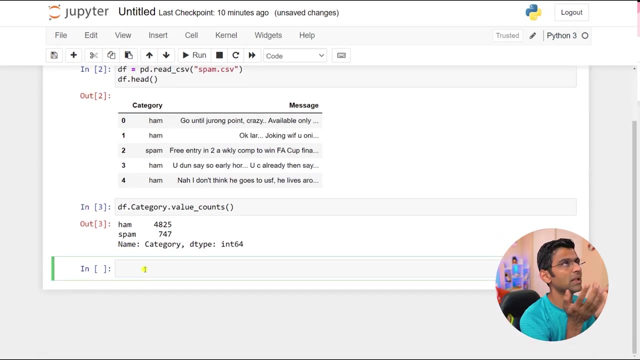 which is a column in a data frame. there is a matter called value counts, and when you use that method, it tells me that there are 4,000 regular email which are not spam and more than 710 spam email, so it looks like an imbalanced data set, but it will still try to explore. 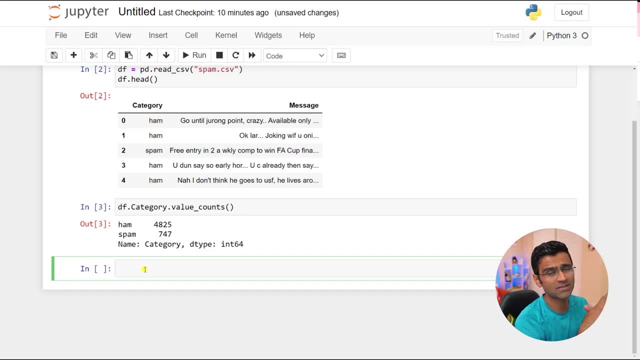 building a machine learning model without handling the imbalance in the data set, and we'll see how it goes. so since this band and ham is entvessed, first I will create a new column, red force for spam. i will have the value of that, that column as one, and for other emails it will be zero. 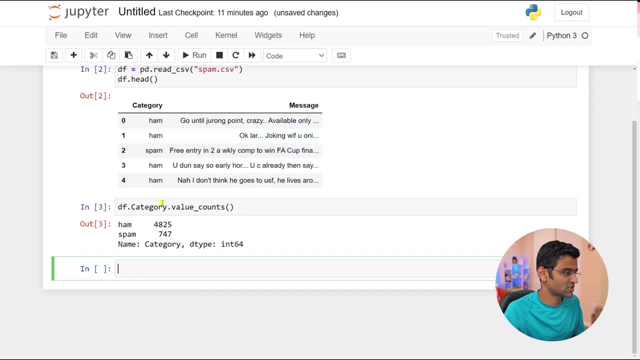 okay. so i want to create that numeric column that can represent spam and ham and the way you can do that in pandas, you probably all know that you can. you can create a new column by doing this and you can say df- dot, category dot apply. so what this will do is, on a category column, it will apply. 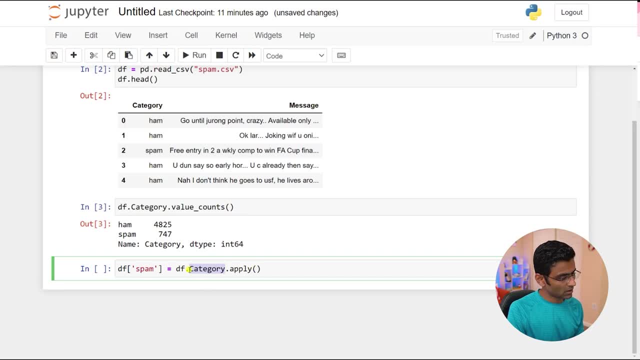 some transformation and it will generate a new column. now, obviously, you can write category column this way as well. i'll just be consistent here, and here you need to supply your transformation function. now, if all of this is japanese is to you again, i recommend you watch my pandas videos and you'll have some understanding here. 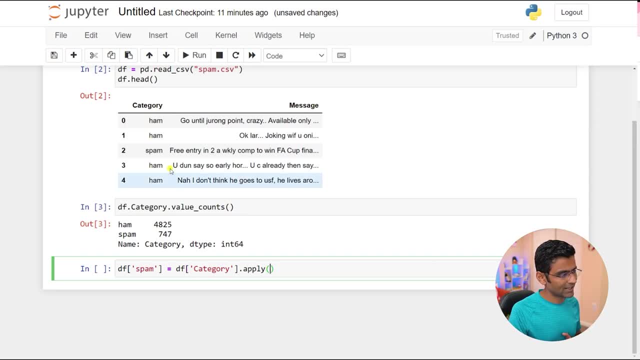 i'm going to write my transformation function which can convert the text into numbers. okay, zero one, and we can use python lambda. so lambda is simple. lambda x means for each of these values in this column. do this, what do you want to do? you want to say: 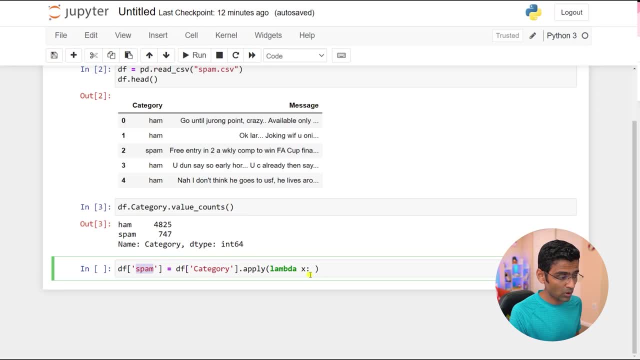 the value of this new numeric spam column is one if x is equal to spam, else zero. okay, you can write a python function as well. you can say: get spam number and you can supply x. you can say: if x is equal to spam, you can return one. otherwise you can return zero. you can do that, this, and instead of lambda you can. 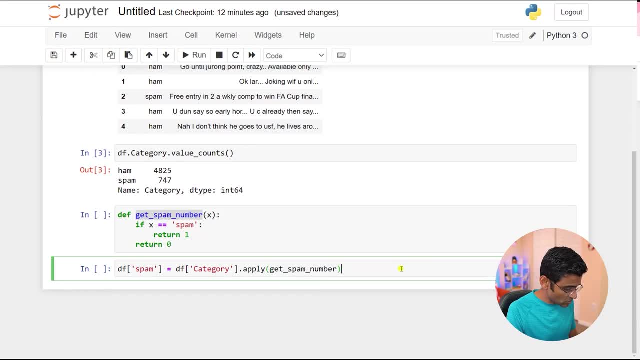 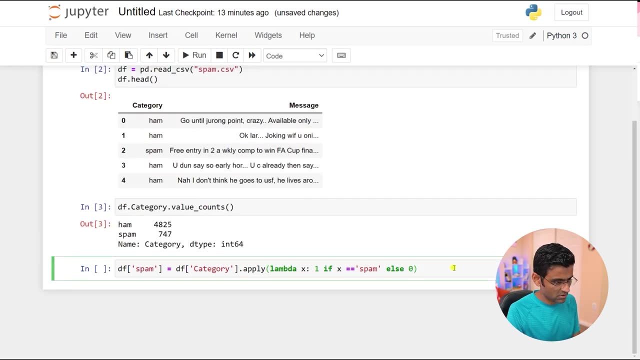 have this method here as well, but these two are same essentially. you know this lambda is just a short way of writing this same python function and when you hit ctrl enter, by the way, you can hit ctrl enter to execute that shell. if you hit shift enter, it will execute that cell and create a. 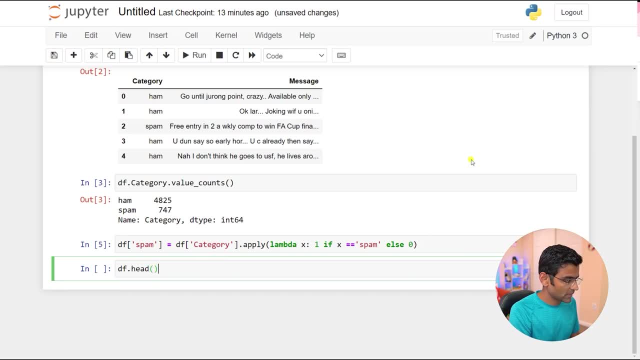 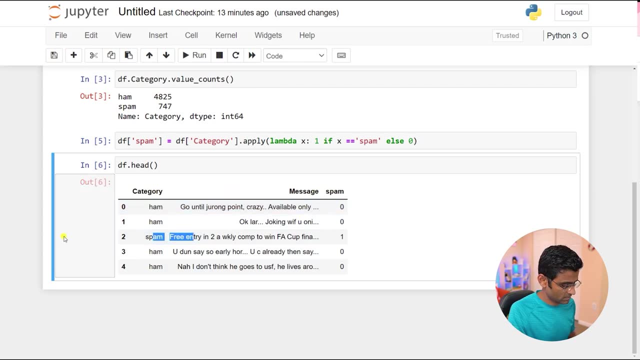 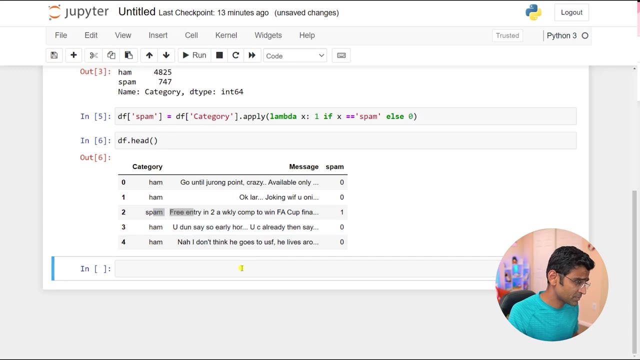 new cell for you now see, spam column is created. you know, whenever the value is ham, it's zero spam, it is one. all right, that's loud, that sounds good. I'm going to now import train this split method from a skill on. this is something we have used a lot during my machine learning videos, so go watch it out. if 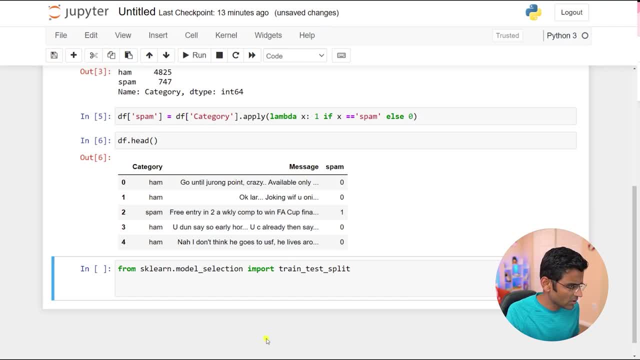 you don't have an idea, and we will be creating training and test data set so we have independent variable which will be stored in X. Y is the dependent way. X is a dependent variable, Y is an independent variable. basically, X train is nothing but the message itself. okay, and Y train, Y, basically, X is a. 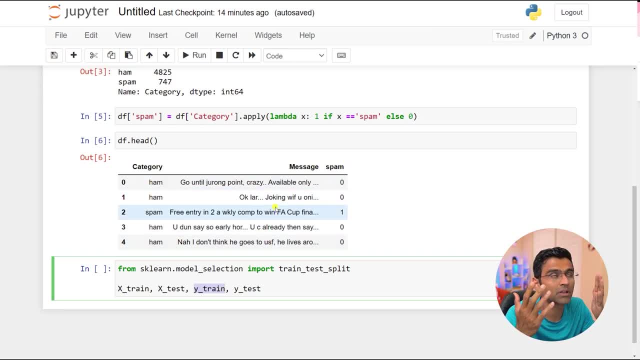 message Y is spam. right, we are determining the- whether message is spam or not- based on the message body. so message body: is your X spam or non? no, spam is Y, okay, and we always split your data set into training and test so that when you are doing prediction, when you are evaluating the 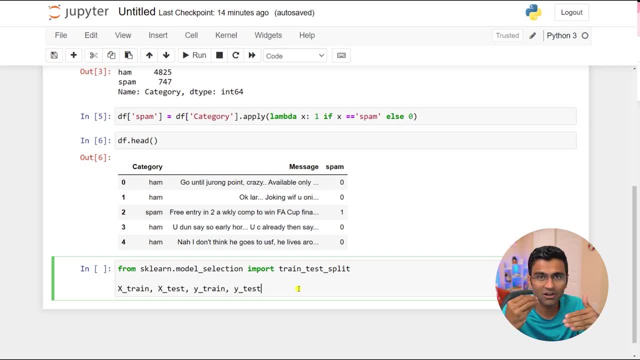 performance of the model. you can use the unbiased sample. you will use X test and Y test so that the model is not biased. we have covered all this theory in our machine learning videos and how I'll be using X train test's. Look to create the split and here you'll be supplying your X first, which is the. 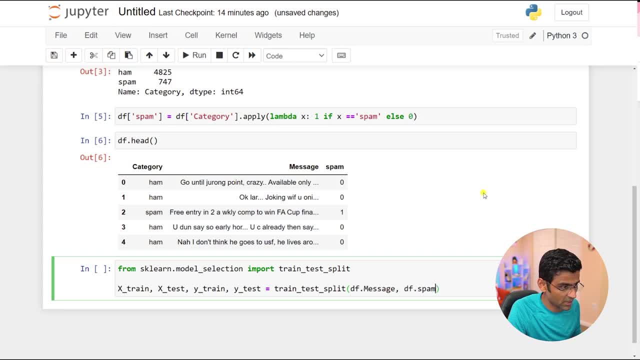 message: okay, and the EF dot spam. this particular column is your Y. you can specify the split. okay, what do you want your test size to be? I want twenty percent of samples to go in my test and eighty person will remain in my training. or in Sistars 10 version Пока, to test your test. You can specify the split. where do you want your test size to be? I want twenty percent of samples to go in my test and 80 percent will remain in my training. atmosphere and process. if you didn't already at all parts, so we do. so. we're going to glorify it and experiment with your training. 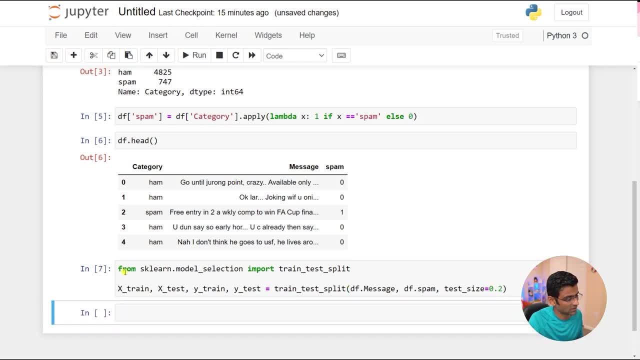 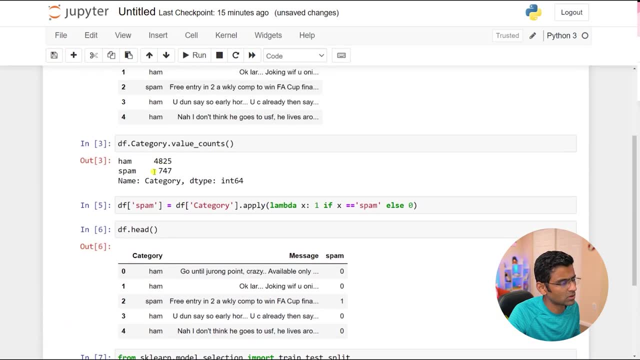 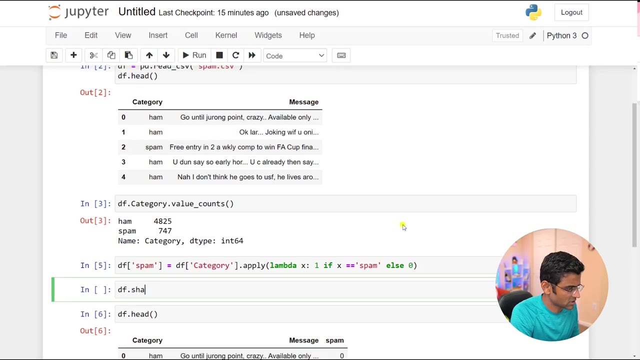 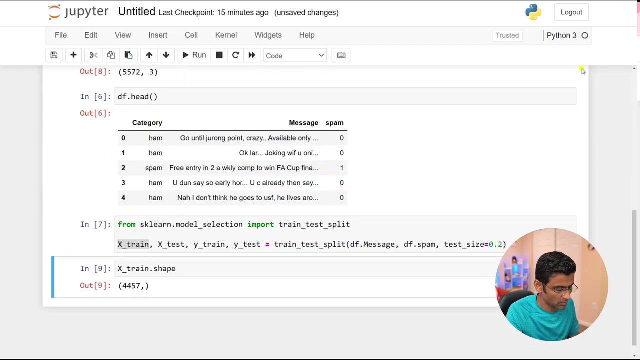 and 80 percent will remain in my training data set. so now you can, you know. see here the total number of samples that we had. uh was. let me show you df dot shape. we had total 5572 emails. out of that. because of the split, i got four, four, five, seven in my 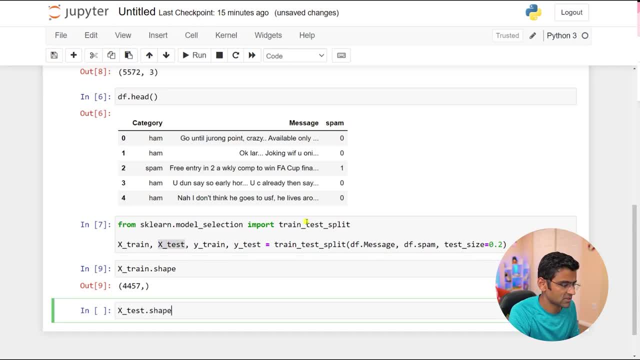 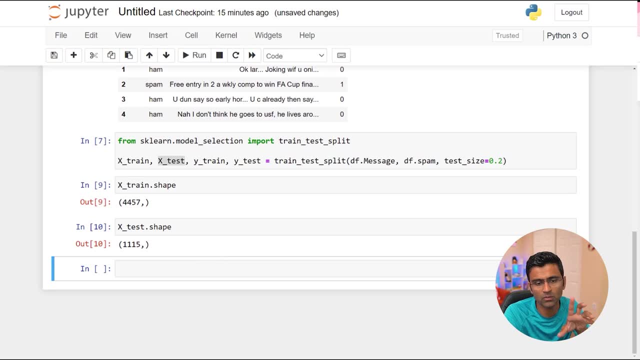 training data set, and my taste is having one one, one point. all right, this sounds so good. now what i will do is i will try to explore extreme. so first of all, we need to train this split. see, you can use this python type function to see what is the data type. 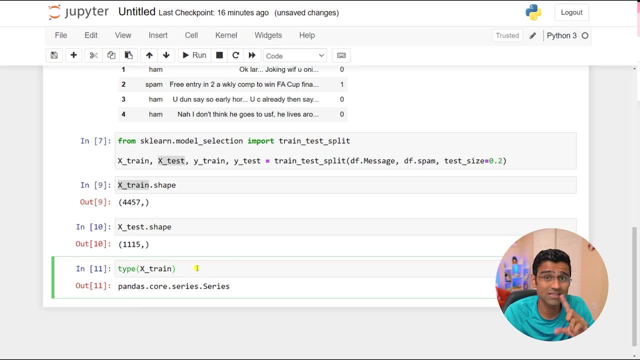 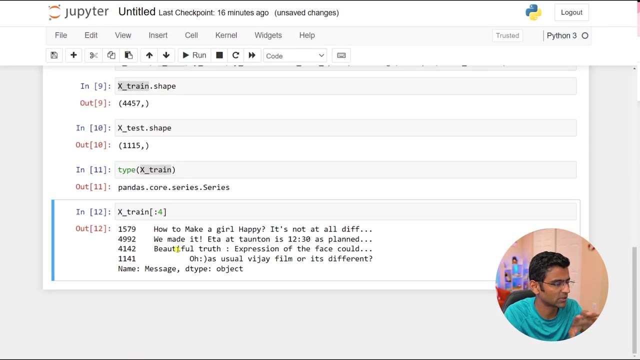 of extreme- variable extreme is actually a series. it is a panda series. okay, and if you explore this thing further, let's say i want to see first four samples. see, it looks something like this. okay, and if you want to see the first email, you can just do this. this is your first email. 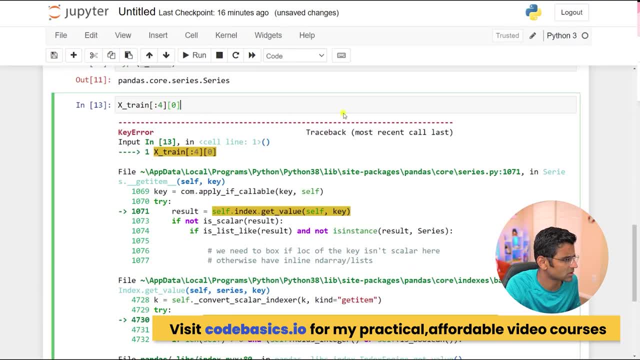 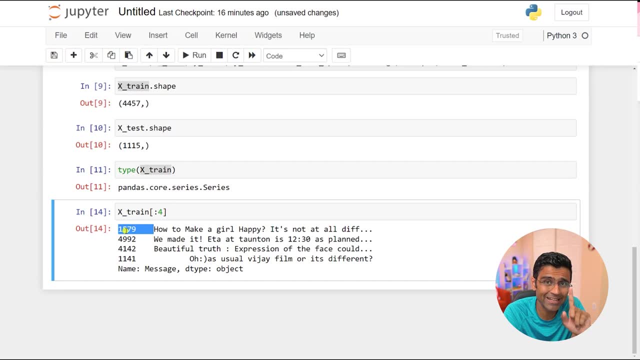 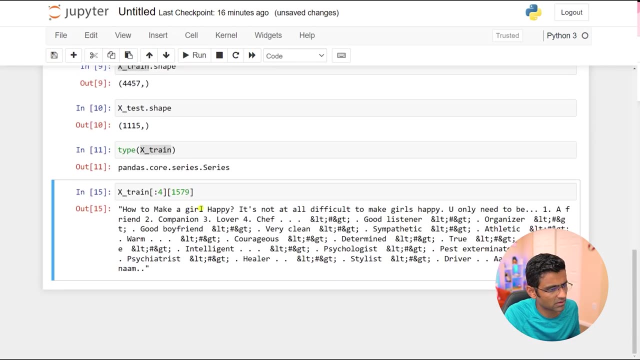 uh, okay, that is not working. because that is not working? i know why it is not working: because the first email, the index, is one five seven nine. see, i mean just this looks like a spam to me. but anyways, you understood the data type of that strain here. now let's see the. 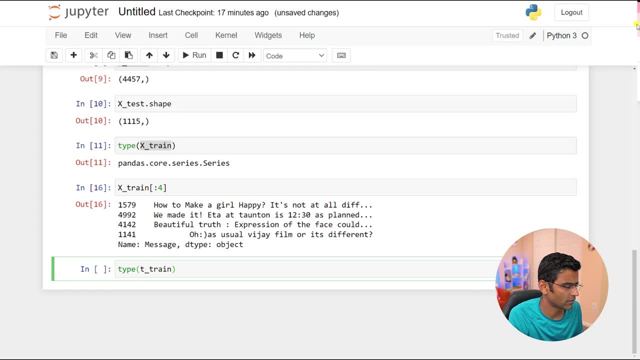 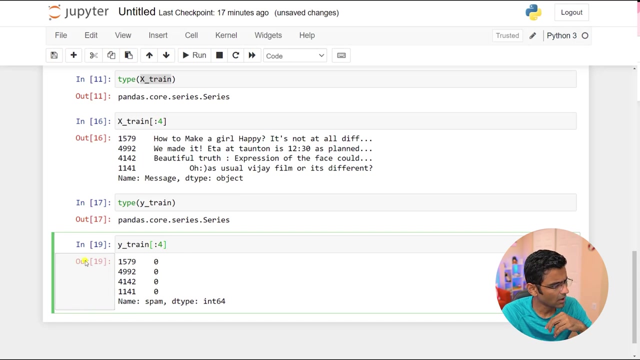 data. take the sample: good job, okay, that was a good sample, oh exciting. y is because capital x, you can have multiple dependent variables. so this could be your table with multiple columns and usually y train is just one column, you know. so x train is multiple columns, y is one. therefore we use capital x and small y here. that's just a convention, that. 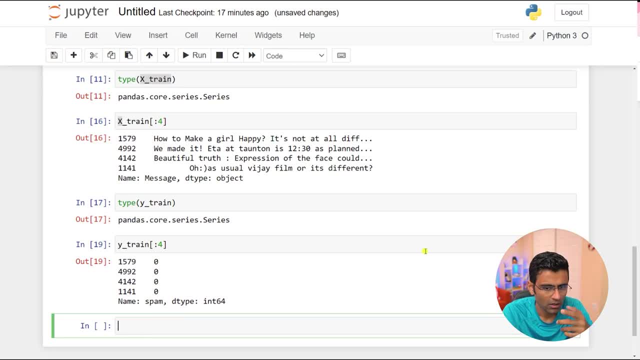 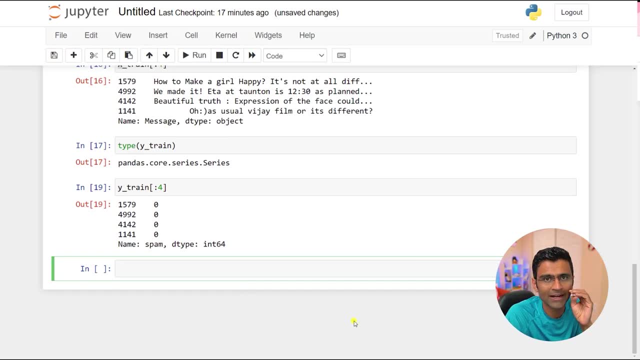 everyone follows. okay, all right. now comes the interesting part from sk learn. we are going to import something called count vectorizer. this will help us build bag of words model for our numeric representation, and the way you import that from sklearn is by using this file. okay, you can. 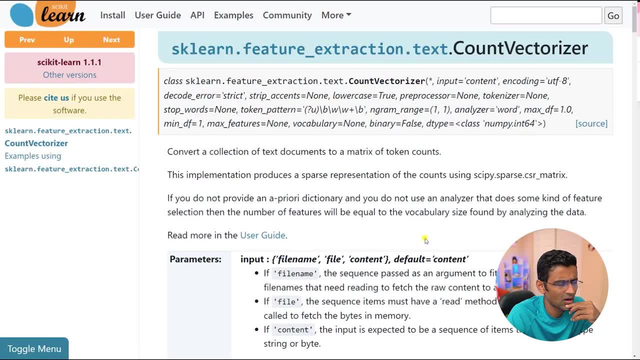 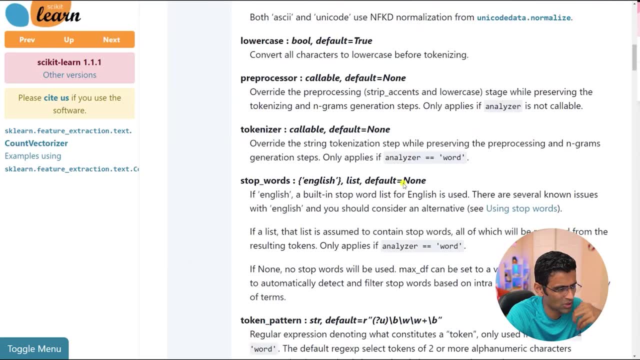 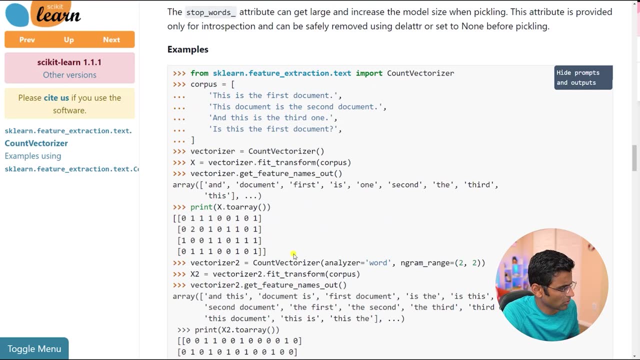 look into documentation. just google sklearn count vectorizer and you will find documentation here. it converts a collection of tech documents to a matrix of token counts. they have given some simple examples here which you can look into, but you already got an idea that it's it's doing. 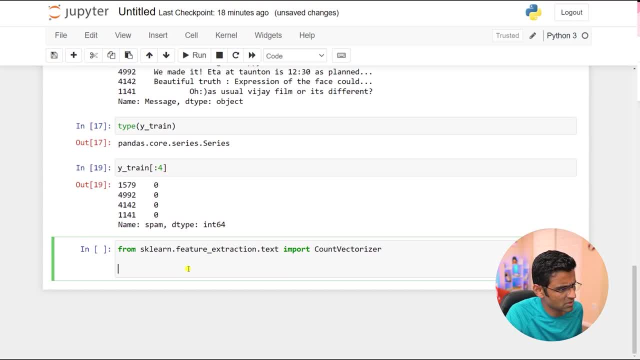 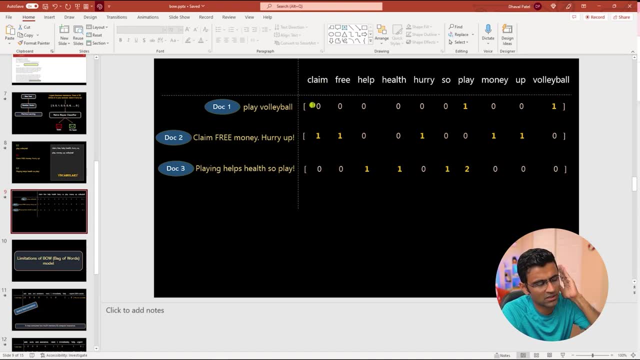 basically what we saw in a presentation, right? so in this presentation, see, it will create a vocabulary and for each of these emails it will have a word frequency or word count at a given position. okay, so by doing count vectorizer, we are generating this metric and each, each of this vector. 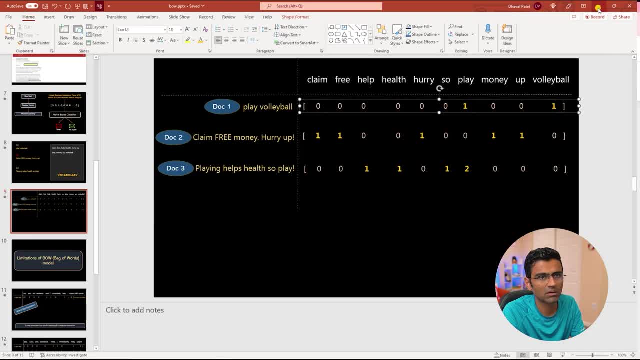 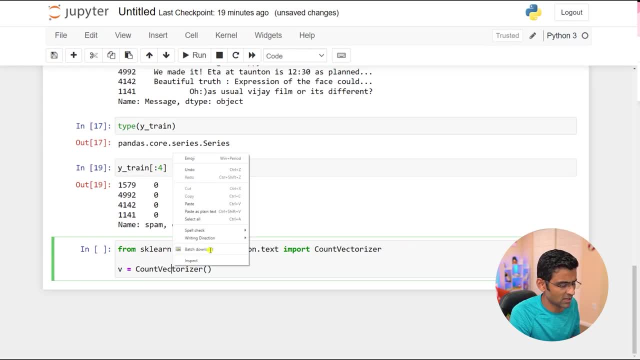 wave. okay, so when you consider all the emails, you get this big matrix. okay, so we will create the count vectorizer is a class and in the python i will create an instance of that class and i will say now, if we, this vectorizer has a method called transform and this transform when you 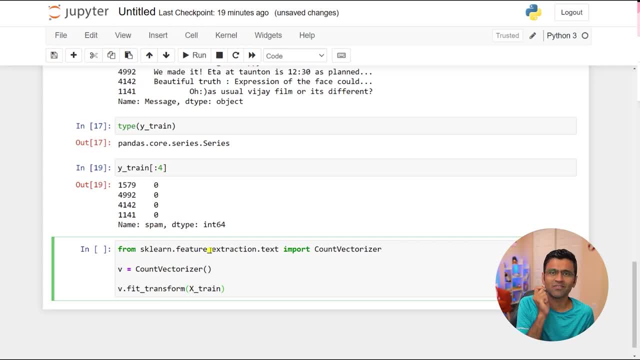 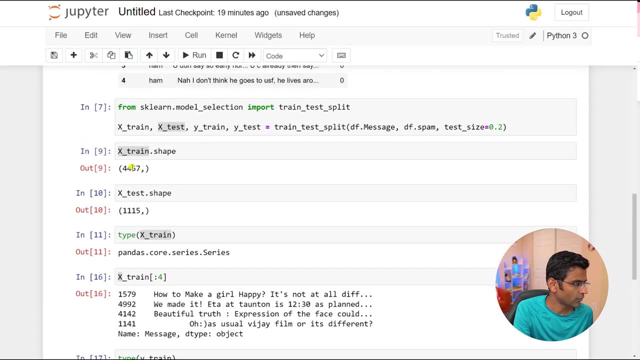 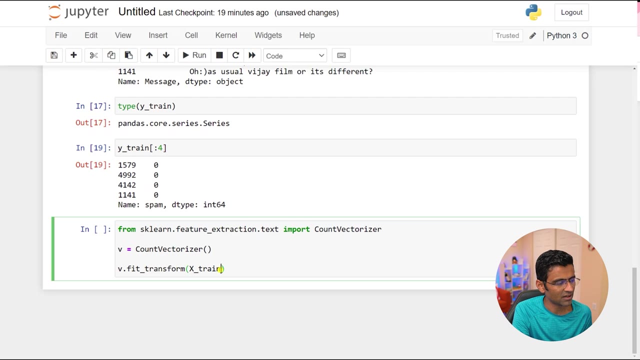 supply your x3. it will now generate the bag of word model for the extreme. so extreme is basically four, four, five, seven emails, different emails, spam and non-spam mix, and i'm for each of these emails. i'm generating the the bag of word model. you have to use values, because that's what you. 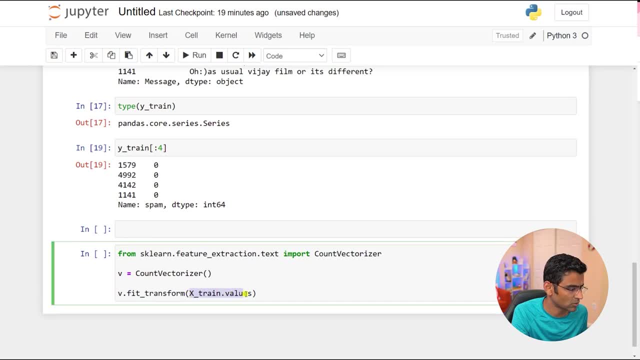 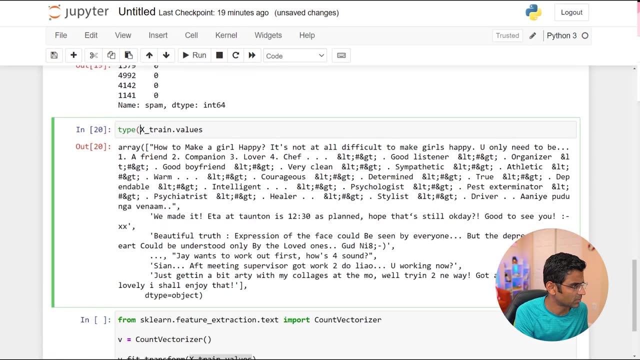 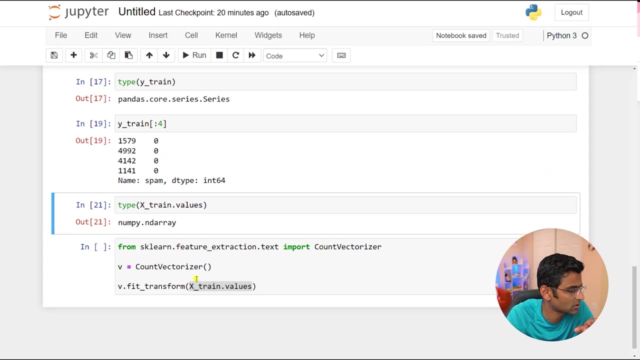 know this expects. so when you do values, it will convert it to numpy array, i think right. so let me just show you, if you do type the numpy and the array and that's what sweet underscore transform expects as a as an argument, so that that's the reason why i'm doing this and you will get. i will call it count vectorizer, so cb. 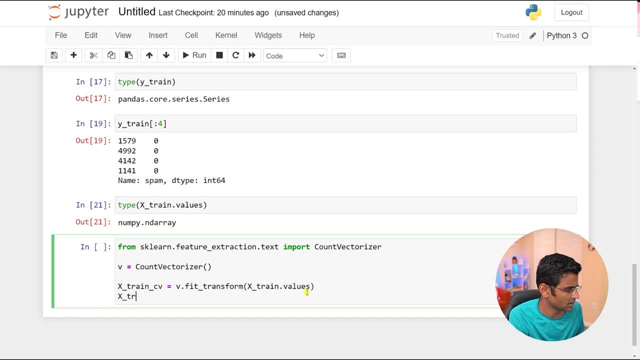 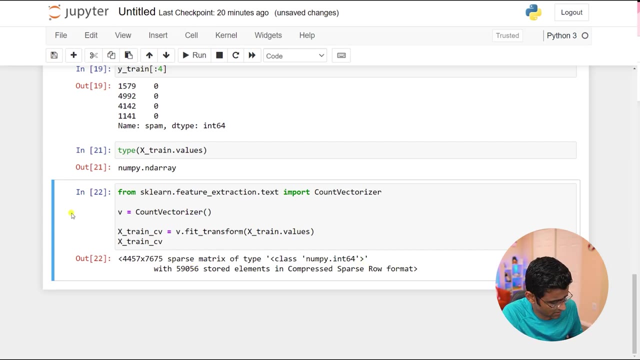 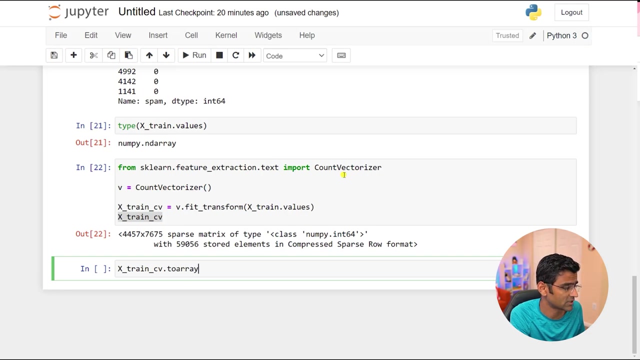 okay, and let's see so once you do that. okay, i got this. it's a sparse matrix of type numpy dot 864.. if you want to view this, what you can do is you can convert this to an array. okay, it's a sparse matrix, you're converting it to. 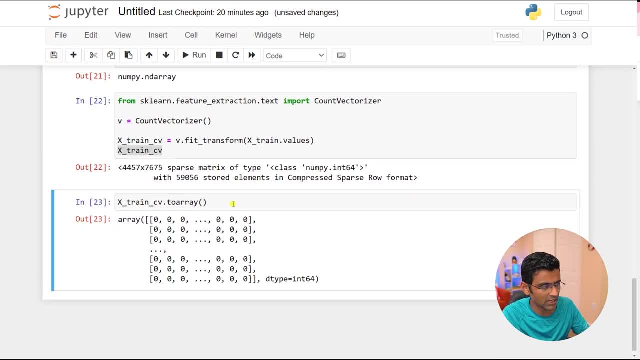 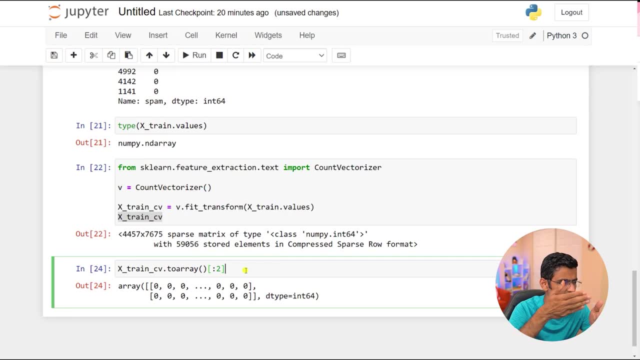 number array. so when you do that, it's multi dimension or two dimensions from a number array. and if you see, look at first two samples- you know they look like this, this: now, obviously this it's a big array, basically it's a sparse metric. so the first sample looks like this: you're seeing zero. the real values are hidden. 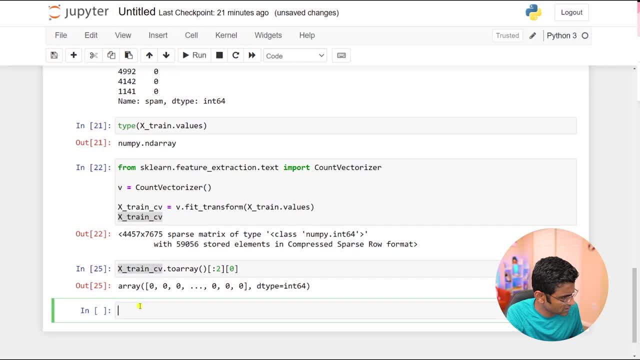 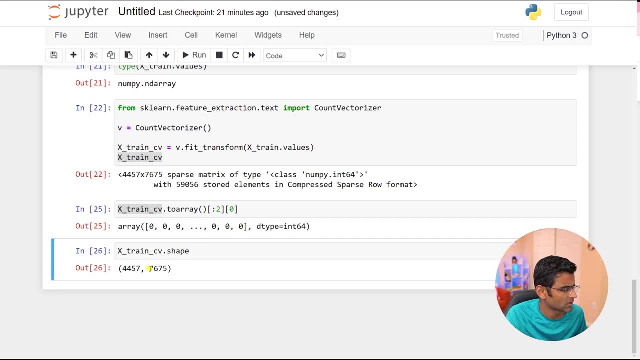 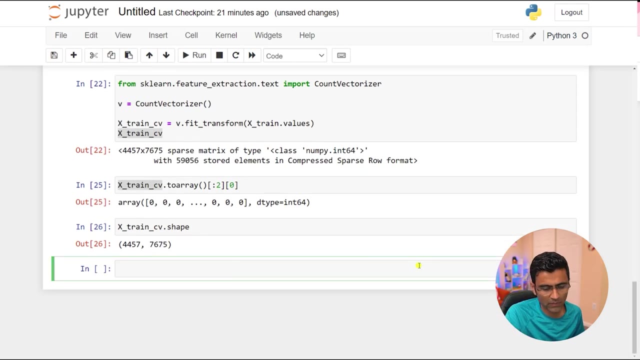 somewhere here, but I want to see the shape of this first. so see, I have seven thousand six hundred seventy five words, unique words, in my vocabulary and if you want to know your entire vocabulary you can use this. this variable V, see V, was found vectorized and if you do, V dot, get feature names out. this will give you. 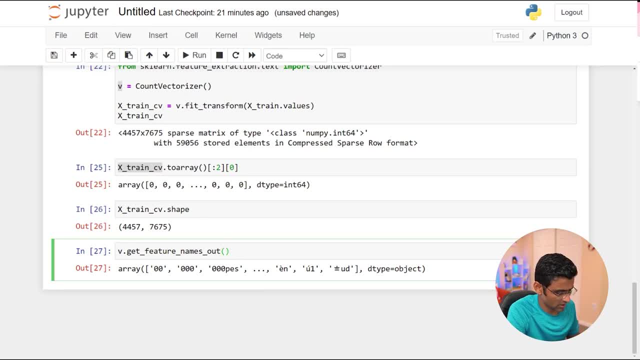 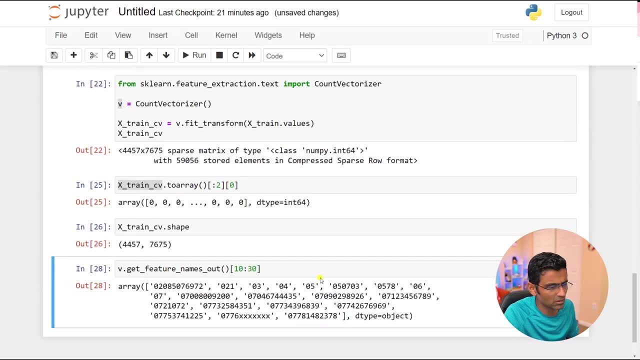 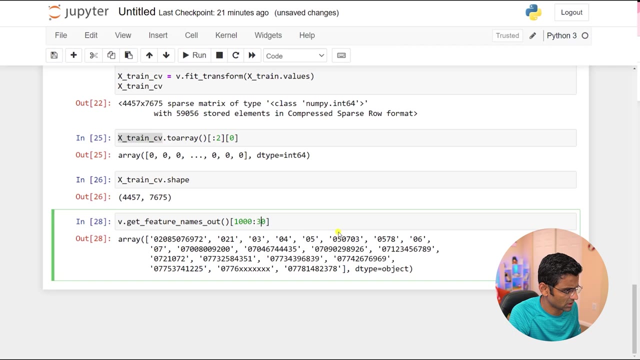 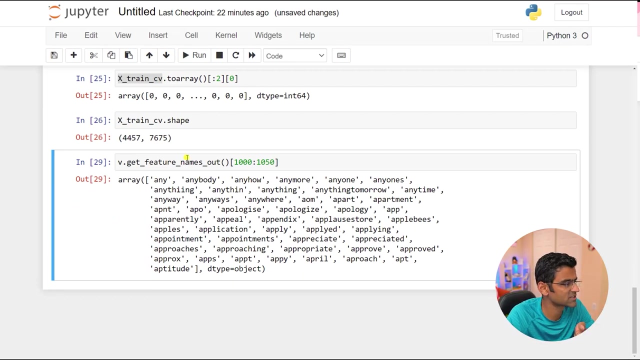 your entire vocabulary. this has all the words. okay, so let me show you some words from this: 10 to 30: see, these are all the words which are present. let's look at thousand two thousand fifty. see, these are all the words that my vocabulary has, and if you 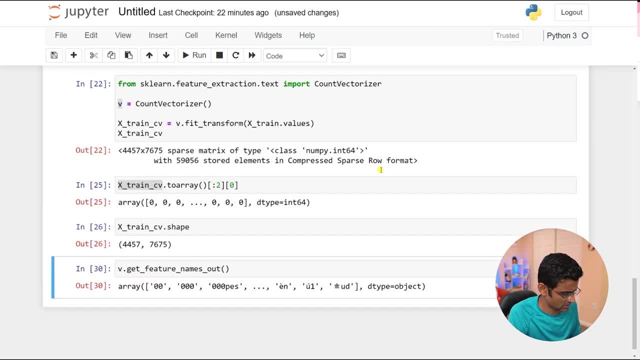 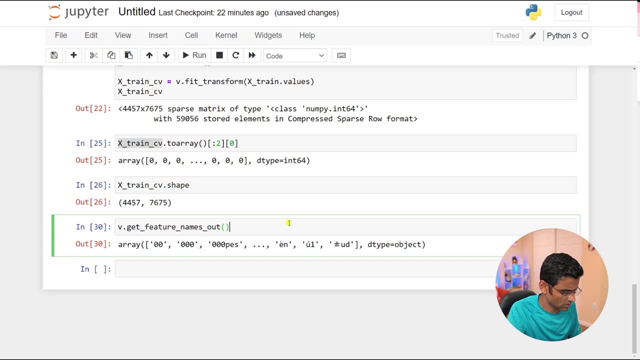 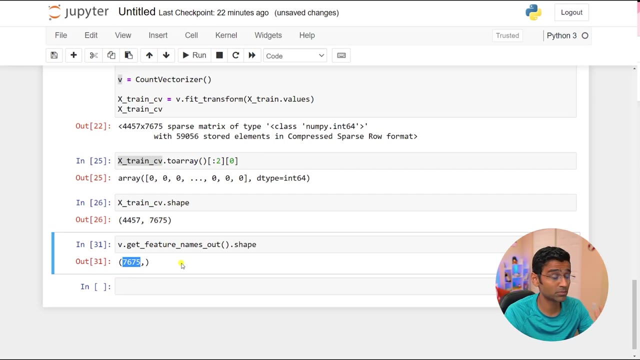 want to, let's see, do the length, okay. so okay, you can do shape and you know seven thousand six hundred seventy five, that's my walkability. folks, now, if you want to know all the methods like, you'll ask me: okay, how do you know what this method? I'll just do dir, read and it will dir is. 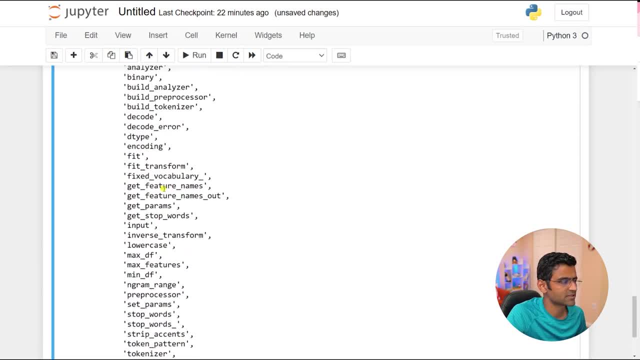 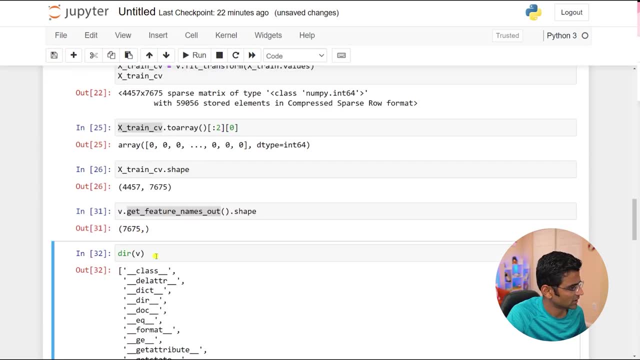 a generic method in Python that can tell you all the methods which are supported on the variables, and I saw this method. I did Google and I found Google is your friend folks. it will tell you the purpose of that method. you can also do read or vocabulary. see, you might have noticed. if you are smart, you might have. 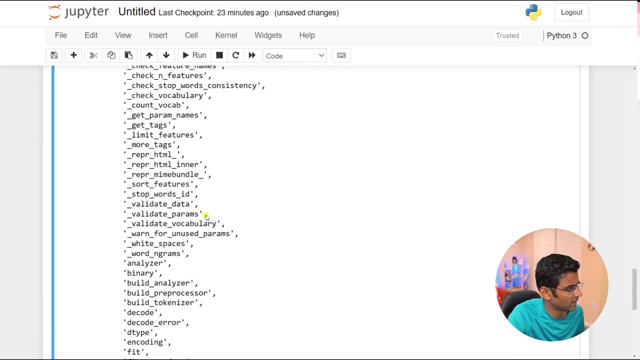 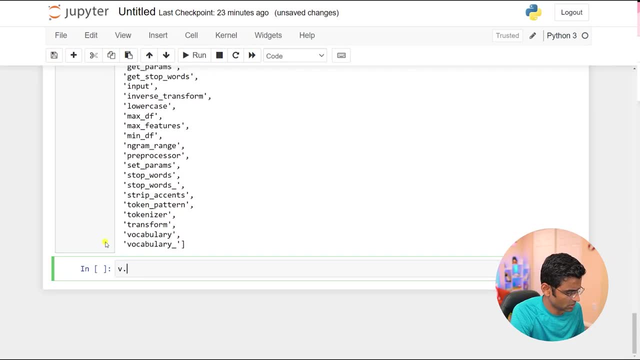 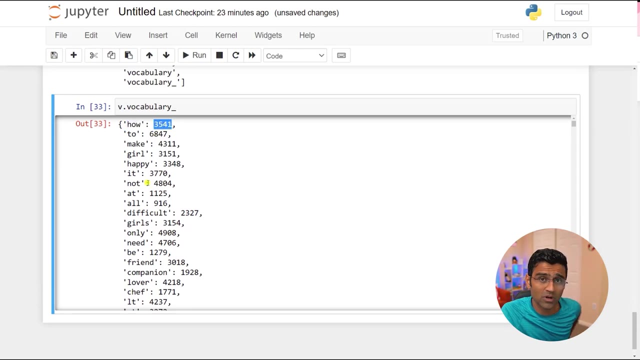 noticed V dot vocabulary, underscore right, that will give you, we gives you the vocabulary. so the world. how is that? position three, five, four, one, so So 3,, 5,, 4, 1 position where? Okay, let me just remove this. 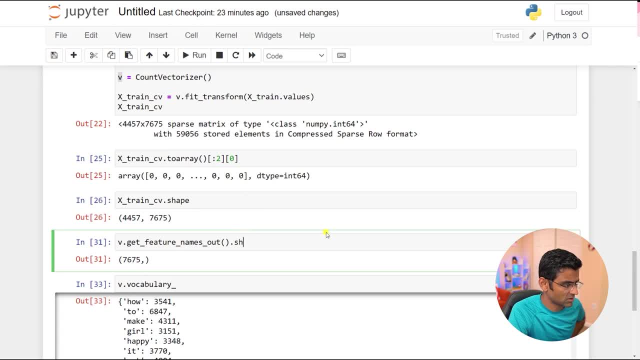 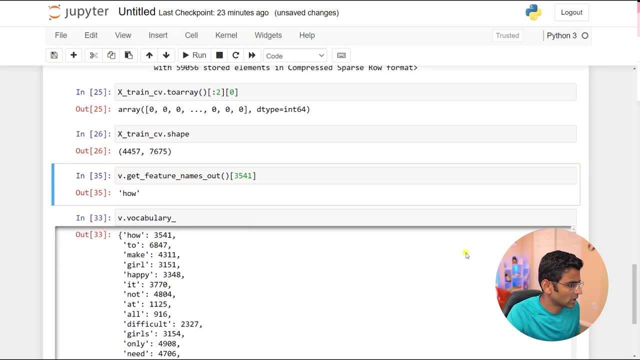 Here in this vocabulary- you see, this was your entire vocabulary- In that if you do 3,, 5,, 4,, 1 position, you get how. If you do 6,, 8,, 4,, 7, you get what. 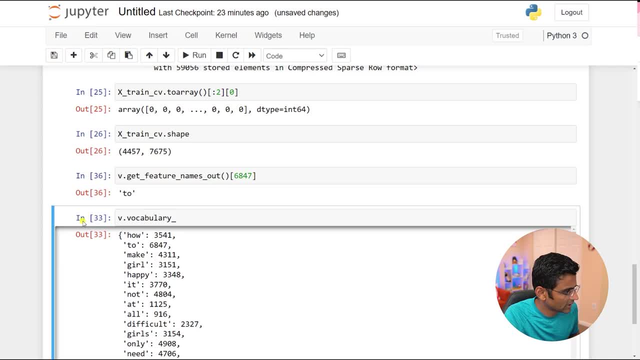 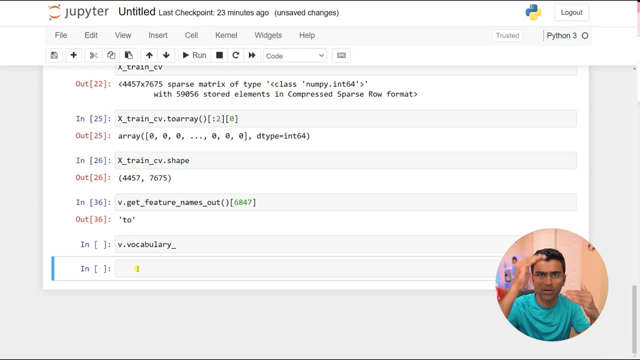 2. See, you just play with it and you'll get an idea. You can also go to sell and you can just clear the output because it's just occupying a lot of vertical space here. All right, So I have 4,, 4,, 5, 7 emails. 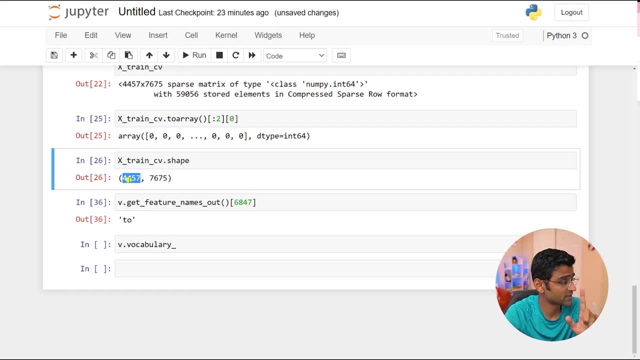 Each email now is a vector of size 7,, 6,, 7,, 5.. Okay, So let me look at my first email now, And what I'll do is see when I look at my first email. okay. 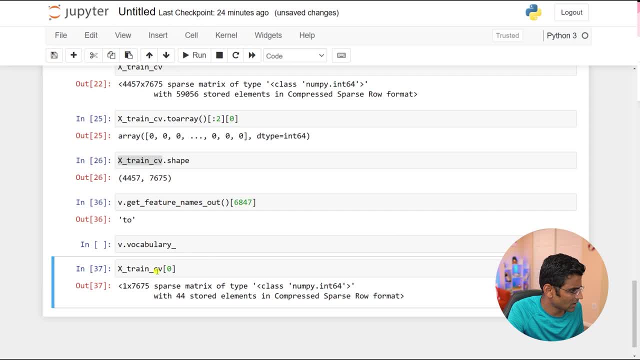 this is my first. Okay, Actually, this is not my first email. I need to. you know what. I'll convert this into a numpy array because this matrix is not good for me, So I'll just do this: convert to array and X chain and P. 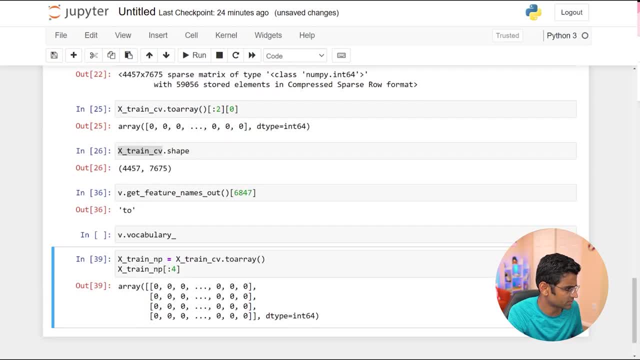 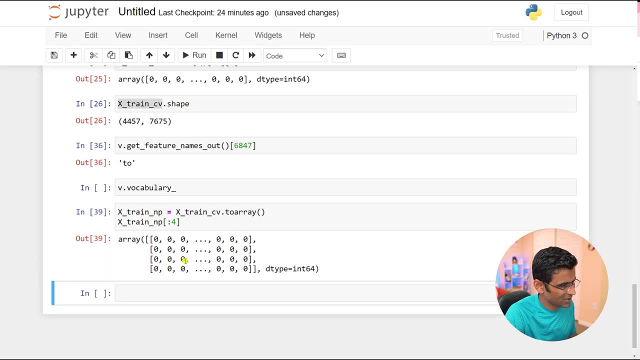 See, this is my numpy array, and the first four emails are like this. Now, I'm just curious, You know what? Because I'm seeing just zero. and I'm curious, what is the vector representation of this email? So one thing I'm going to do is, since majority of these values are zero, 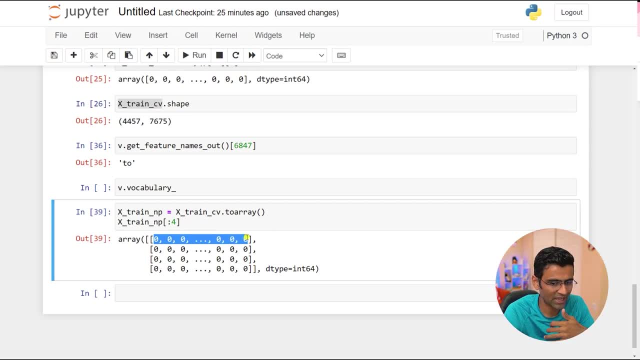 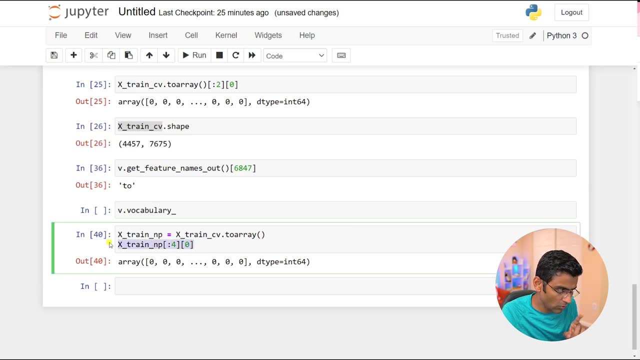 I want to know where is non-zero value, And you can do that by see. let me look at first email. Okay, So this is my first email. I want to know the index where there is no zero value, And you can do it using npwhere function. 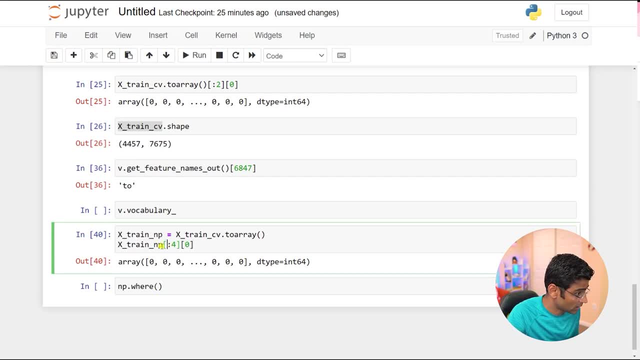 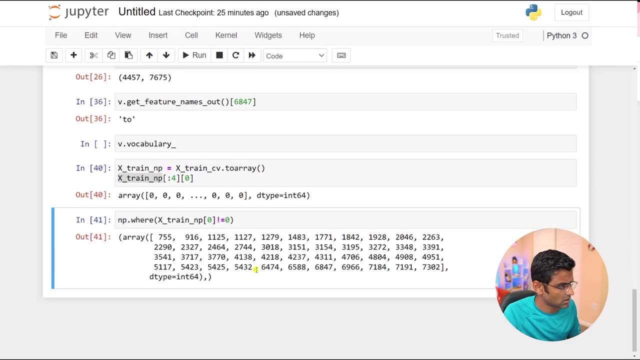 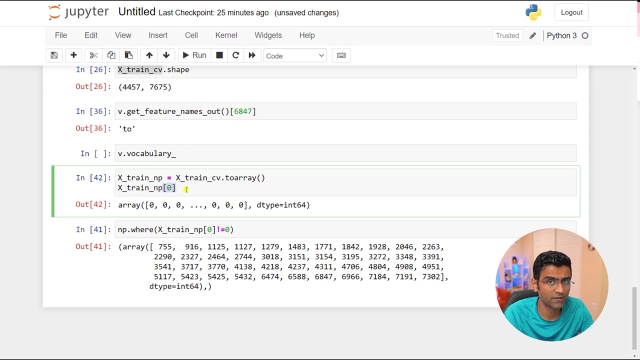 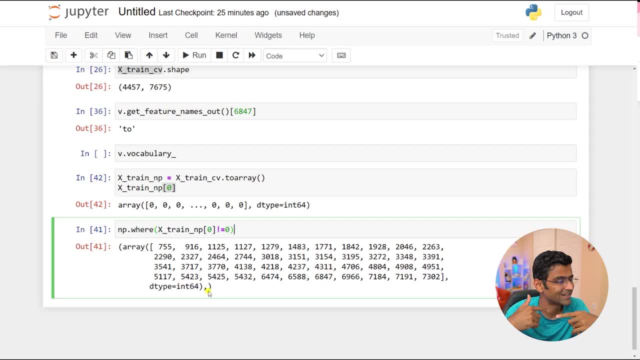 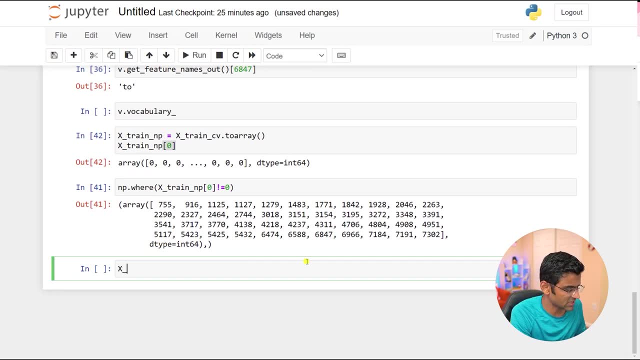 And in that email I want to know what are the indexes where the value is not zero. Okay, Now see what this means. is this? Okay, Let's dissect this step by step. It's not as hard Like if you pause this video thing for a moment. it's not that hard. 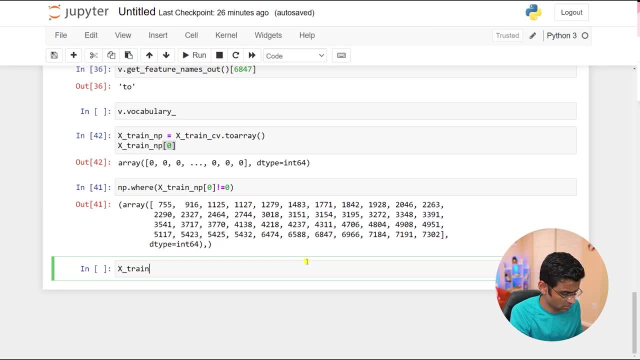 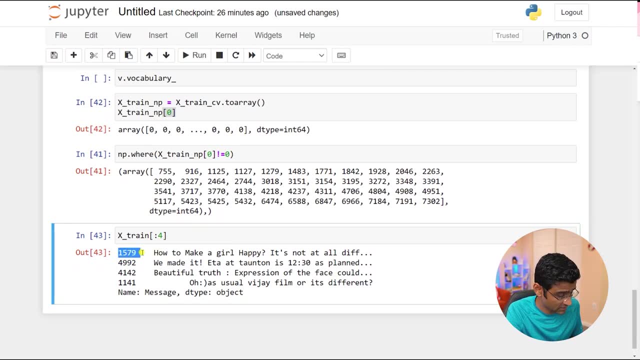 Okay, So X chain, your X chain In your X chain. the first four samples were this: Okay, And the first sample is this: One, five, seven. That is your first sample. It's just the series index. 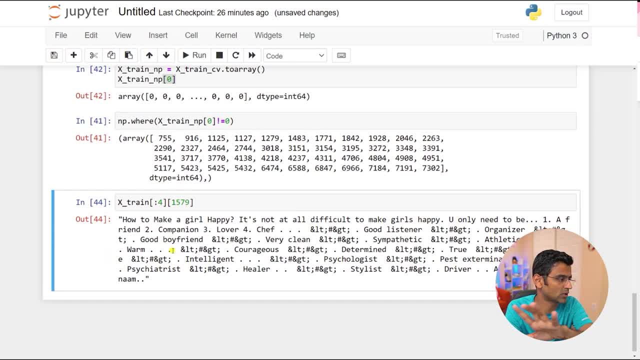 So you have an email that looks like this: Okay, And when you converted this into a vector, basically what you got is at 755.. So now, where is my vector? So that is my vector. Correct, So this is my vector. 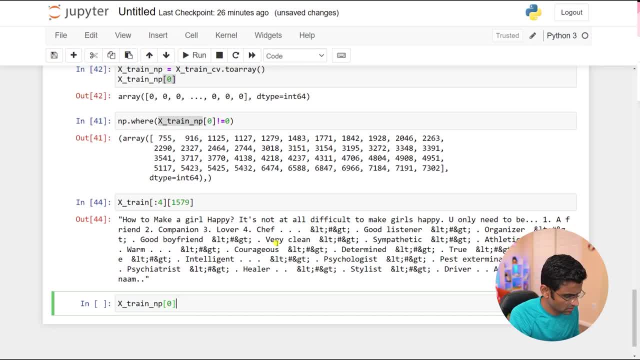 Okay, And for this vector at 755 position, I have a non-zero value. So I have one value right. Then other one. this one, 916, is non-zero. I'm just trying to find a value where it is not one. 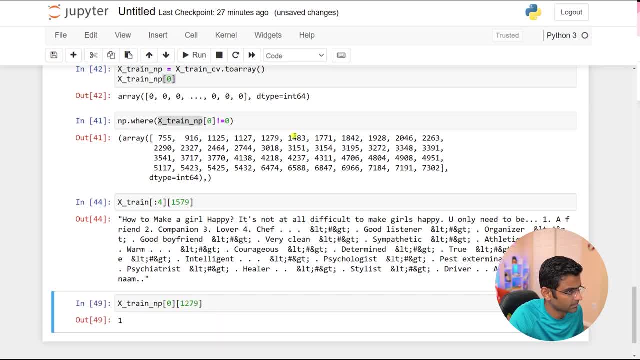 Okay, I think trial error is going to take a long time. Okay, Anyways, I can just do this. I can just show you this: 1483.. Okay, So 1483 is one. So what is 1483?? 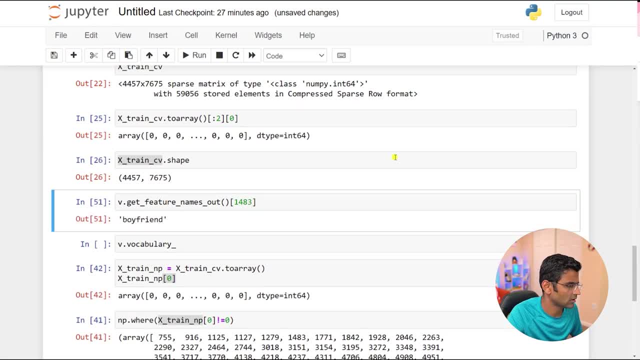 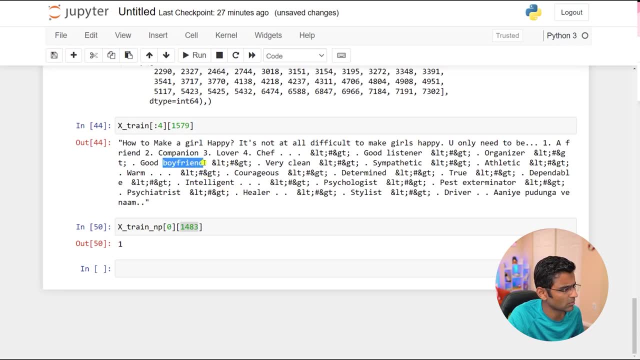 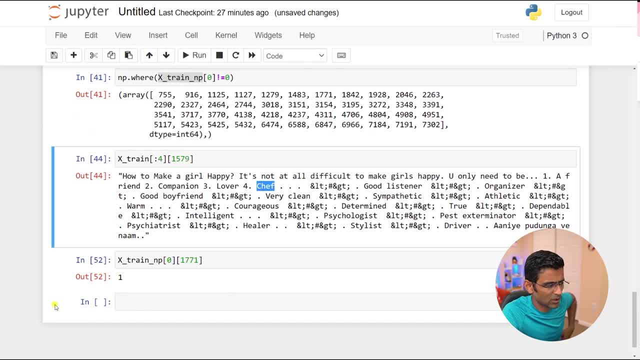 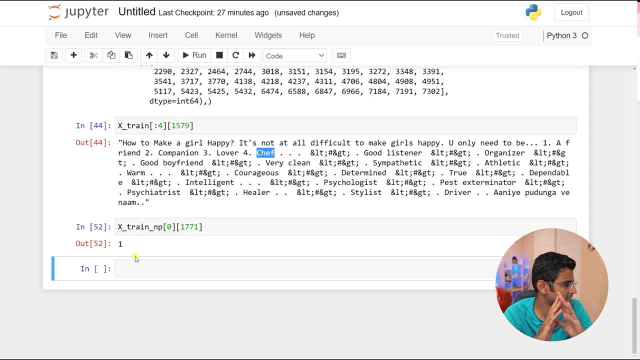 All right, Now I'm all set. My training and tests are ready. I'm all set to build my machine learning model. Yes, folks, Now we are going to build machine learning model, And the way you do that is: I'm going to import this naive base model. 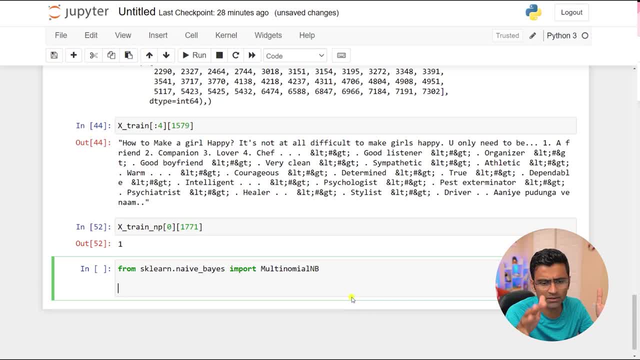 So in naive base, there are two models, Okay, Multinomial, Multinomial- And there is another one, So we are going to use multinomial. If you want to see the difference, understand the difference between these two. 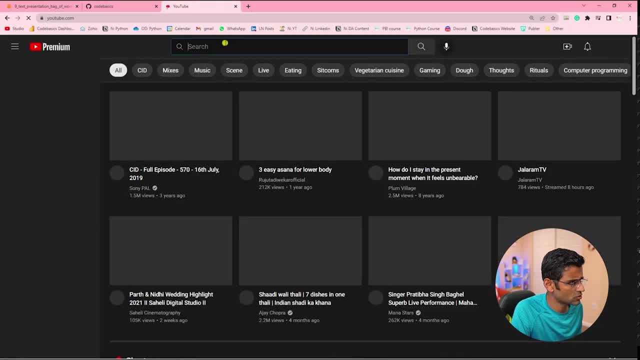 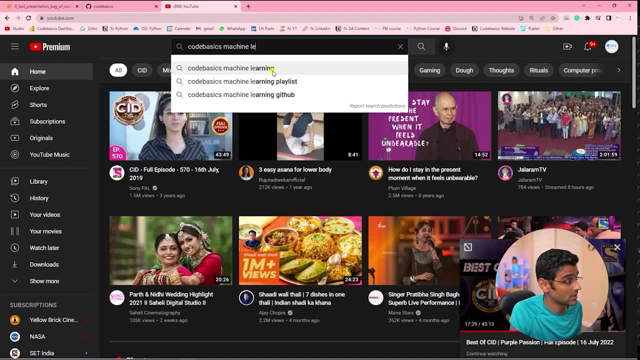 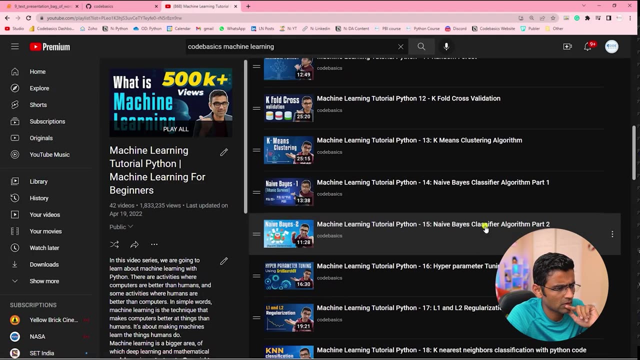 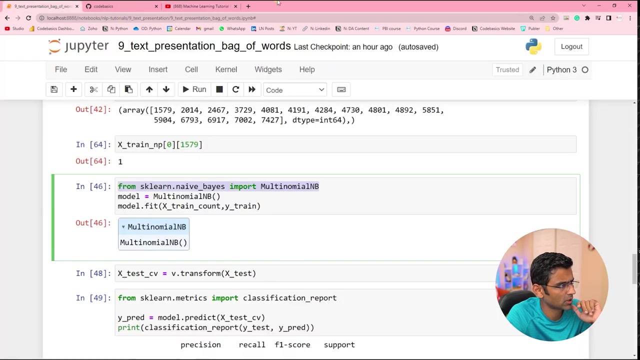 you can go to this website called YouTube search for Core Basics Machine Learning. See, my wife likes to see CID. So Core Basics Machine Learning. In that you know we have called naive base these two parts, So if you watch these two videos you will get an idea of what I'm talking about. 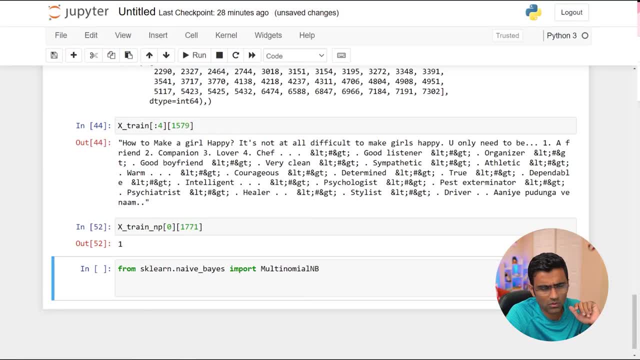 Okay, So now I'm going to create a model by using this multinomial class. And see, training machine learning model is as good as calling fit. You're just calling a fit method. here You will say X train, C, V, Y train. 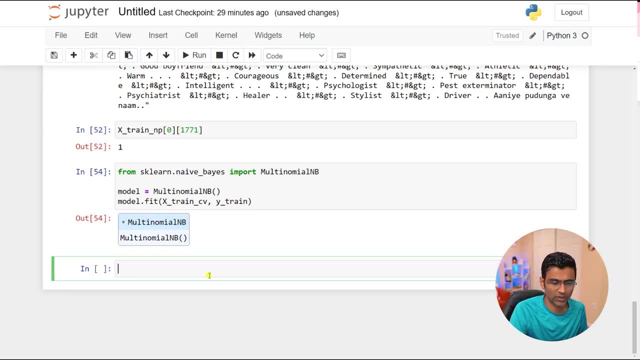 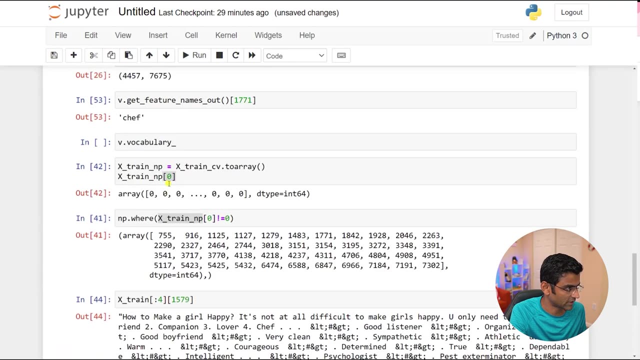 Okay, And when you hit control enter, actually train the model. And now I want to evaluate the performance of the model And the way you do that is, see, you need to use the vectorizer that we use. See, V is count vectorizer. 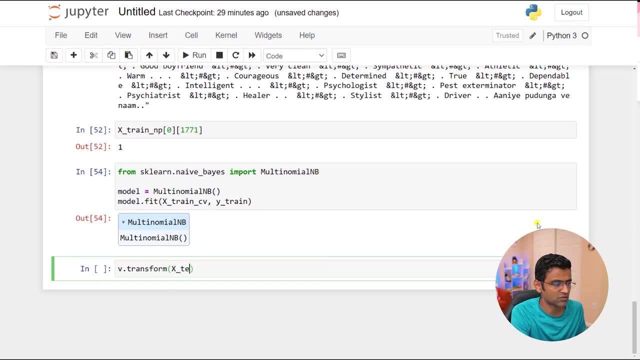 Using that count vectorizer. we need to transform X T. Because X T Is simple email, right Word email, You need to convert it into count vectorizer first, In that by doing that you will get count vectorizer for X. 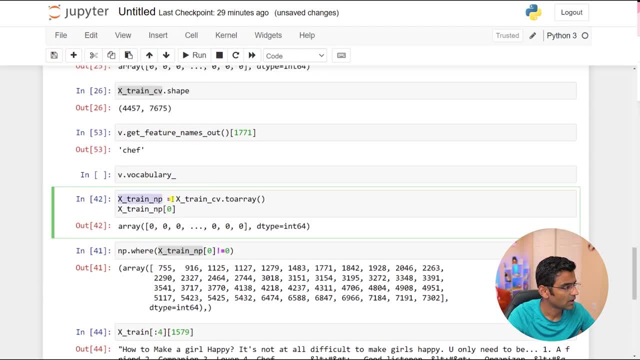 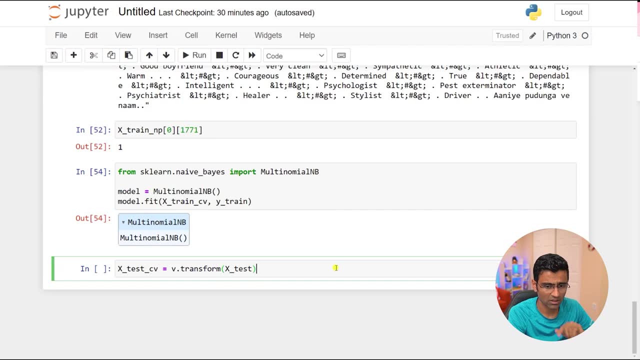 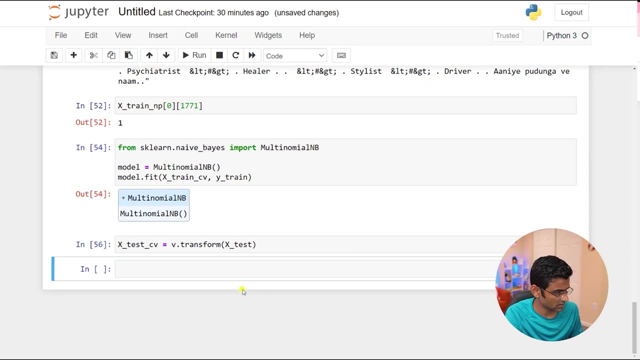 T C V. Similar to how you created X train CV, I'm creating X T C. All right, And then you can, For evaluating the performance Of the model, you can import classification reports from SK. 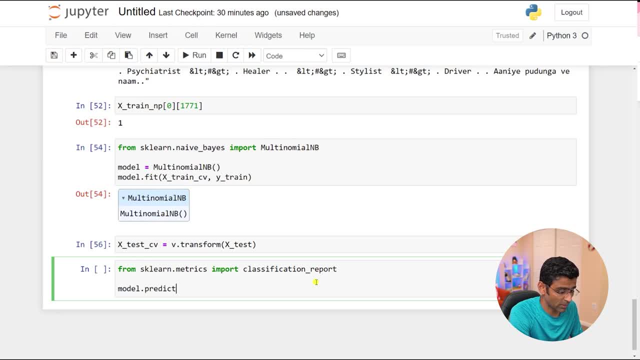 Learn And you can say: okay, now, model, do predict. So my model is trained at this line And now it is ready to do a prediction. And the prediction it wants to do is on X taste CV, And whatever the result you will get, we'll call it Y prediction. 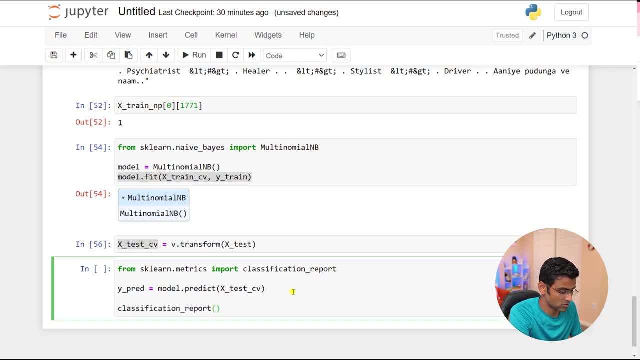 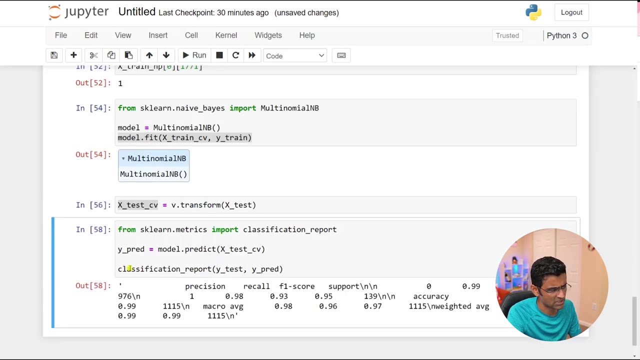 And the way classification report works is you first give the truth, which is your Y taste, And then you give your prediction: Okay, Okay, And when you do that, You will get this. And if you want to do pretty printing, if you use print method, you get a nice layout. 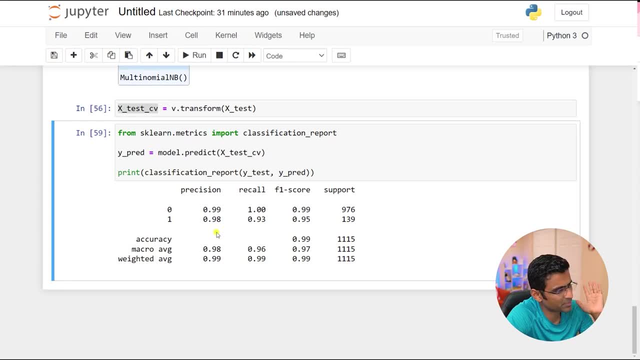 Now folks look at the accuracy- See precision, recall for both the classes, spam and non-spam. Right, This is spam, This is ham. For both the classes. the accuracy, the precision and recall. they're pretty high. 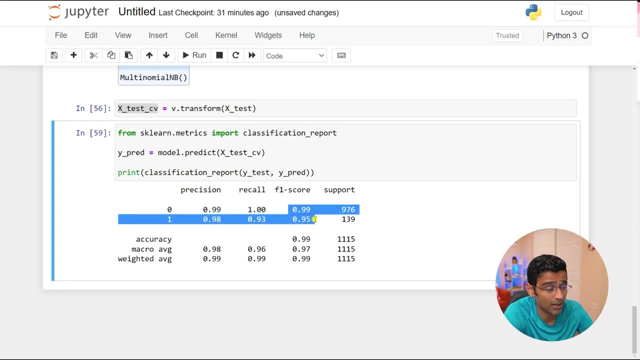 Right, So I will change that to 3.. So the accuracy, Okay, Save, Save, Save. F1 score is high. I used F1 score, and all that because the class was imbalanced. remember our spam emails were very less compared to our regular ham. 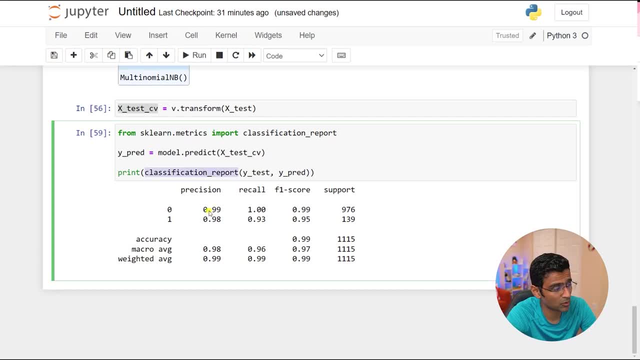 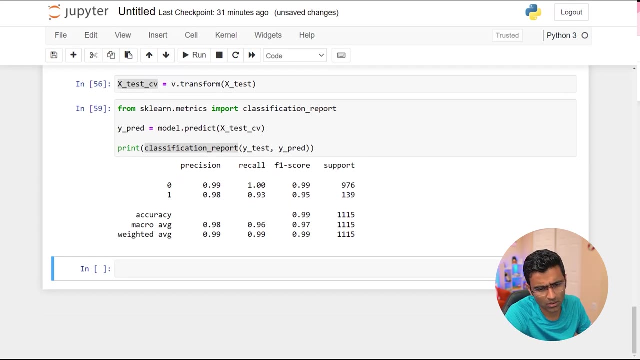 emails and therefore I wanted to use classification report and not just the accuracy. okay, whenever you have imbalanced data set, you need to use classification report. you need to look at F1 score recall precision for all the classes. all right, and I can do some testing on the sample email. clearly the 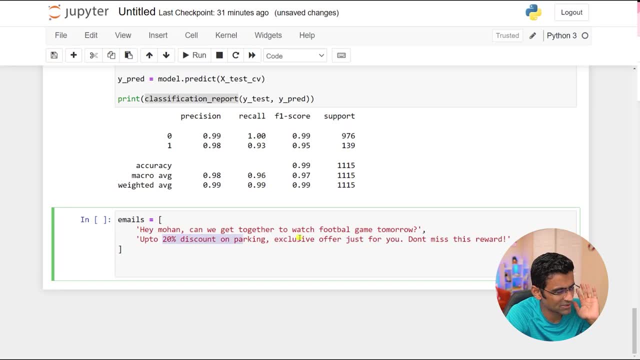 first one is not spam. the second one is spam: see: 20% discount, exclusive offer just for you. who gives exclusive offer to you? see, in this world you don't get anything for free. so whenever you get any email or any scheme, this is a general life philosophy. when, when, where this is free or huge discount, it means it is. 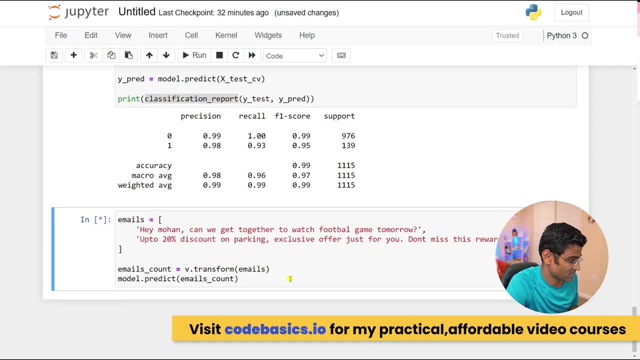 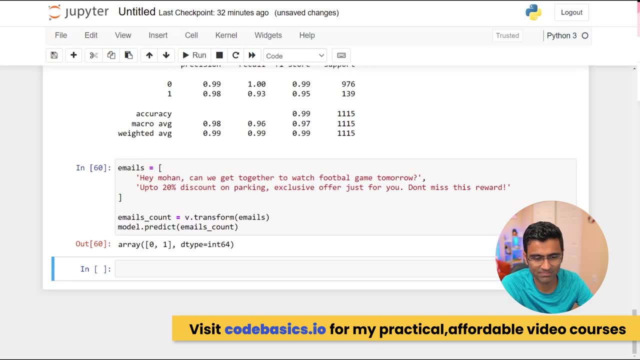 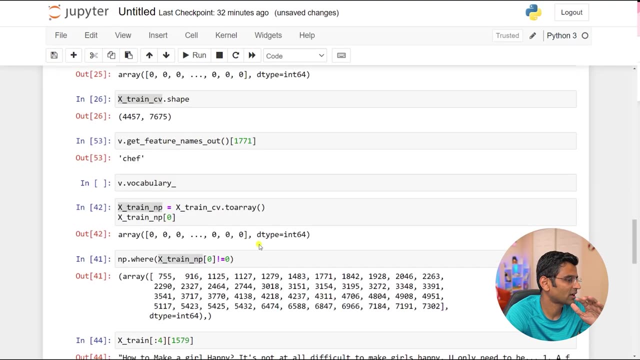 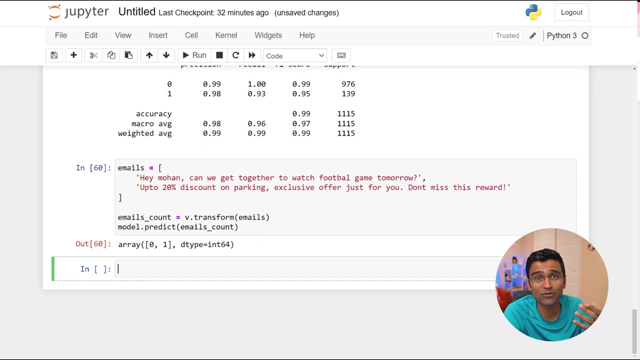 spam when you do transformation. see, the first one is not a spam, the second one is a spam. all right now, see, you did all this work. okay, creating count vectorizer, train display, all of that. will you cry or laugh if I tell you there is an easier way of doing this, using SQL and pipeline? see, I will do the same thing. 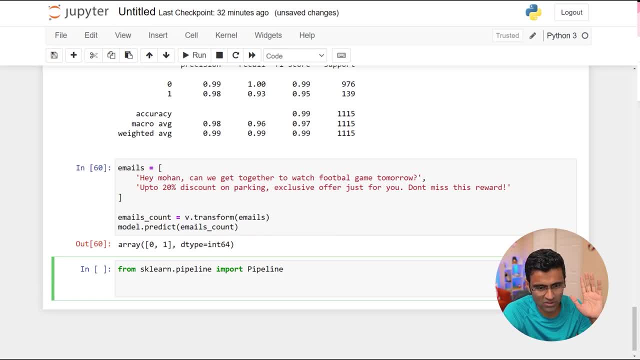 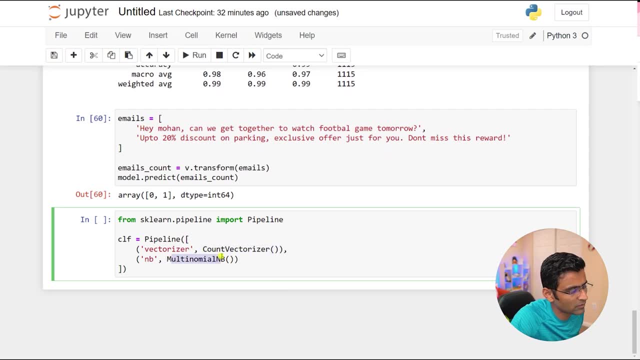 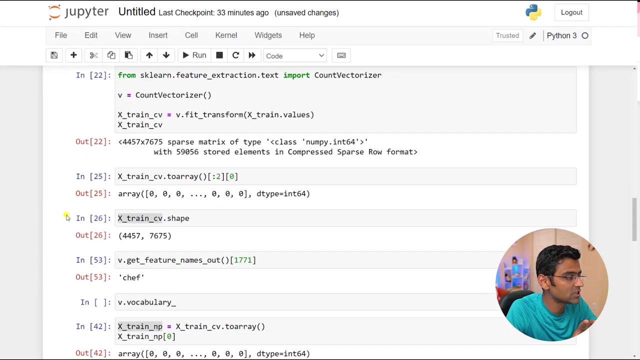 now using SQL and pipeline very easily. so the way you create your SQL and pipeline is by supplying count vectorizer and multinomial be and be, right now base. so if you've seen my machine learning model, you know so pipeline is nothing. but basically, whatever steps you are doing manually, here you are. this is a convenient API. 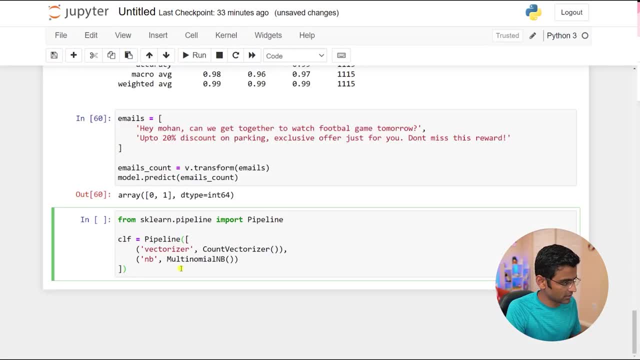 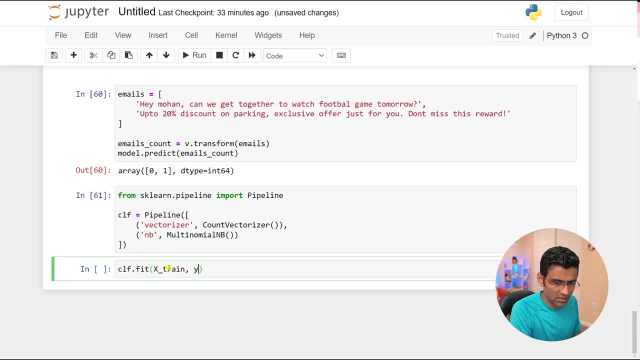 that you can use. okay, and once this pipeline is created, you can just do a few more things like you can do: CLF, not fit X train and I train. see here, I am not saying a strange CV, because the count vectorizer will be taken care of. 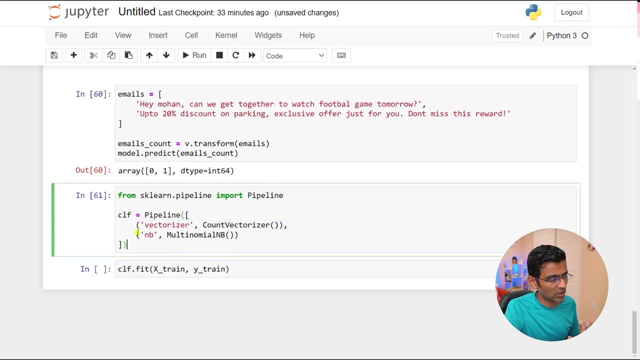 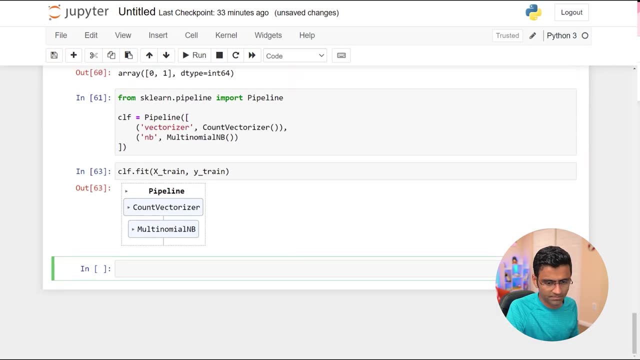 by the pipeline say it is the first step in the car in the pipeline. so now the API looks much simple. you created a pipeline. now you're saying CLF, not straight. okay, and then So I can have my classification report where I will say ytest is clfpredict. 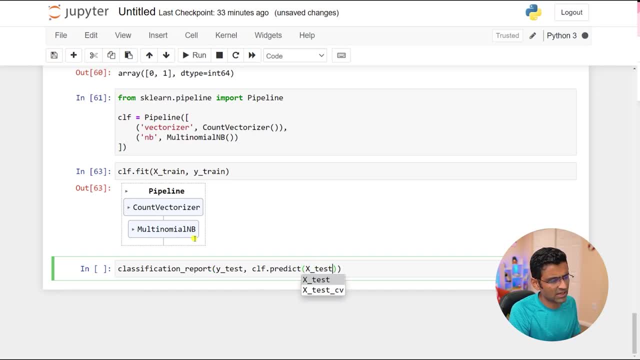 When I do clfpredict and supply xtest, I get that ypredicted right. So instead of saving in a variable, I can save it in a variable too. Here I can say ypred: Okay, This is your yprediction. 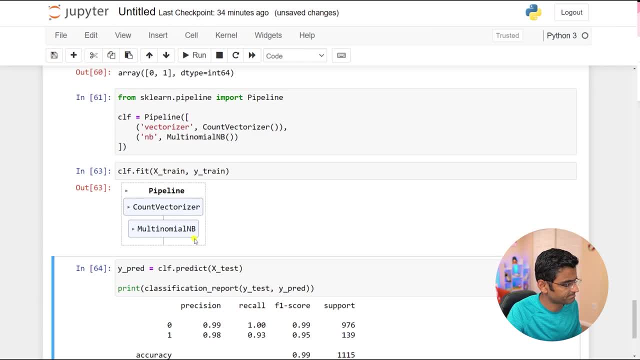 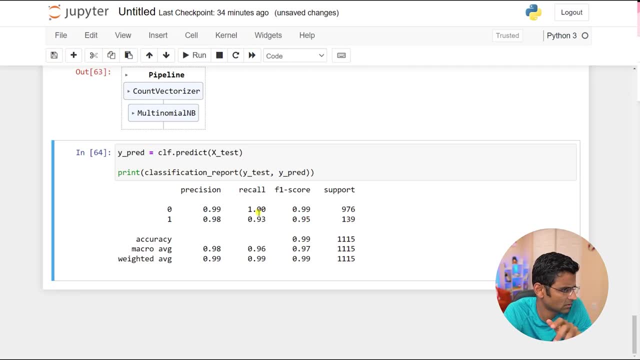 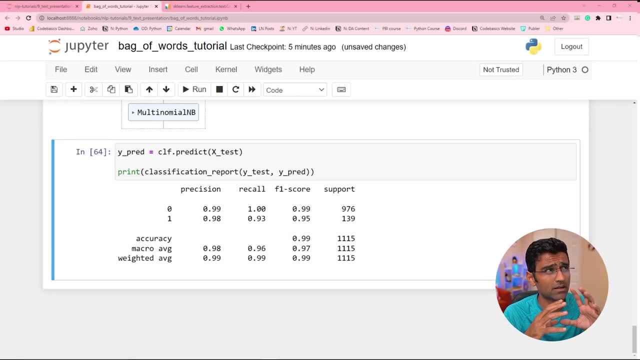 And you print it out. All right. So you see accuracy and the precision recall. everything is pretty good. That's all I have for this tutorial. For exercises, I did not have time to build one, But if you want to contribute and if you want to prepare an exercise for this particular tutorial, 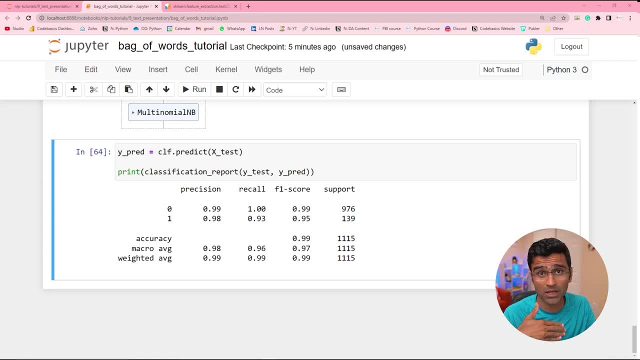 please give me a pull request on GitHub page. Many times when I find time later on, either I or some of the volunteers will prepare exercises for my videos, and it's always advisable that you check video description because you know you will see exercises coming up after a few days of posting this video. 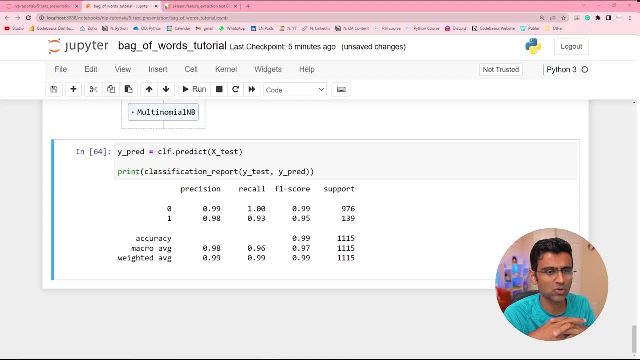 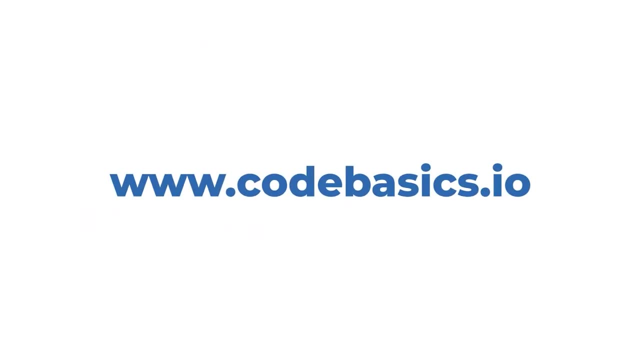 So do check out the video description for exercises. I wish you all the best And if you like this video, please give it a thumbs up and share it with your friends, And I will see you in the next one. Bye.